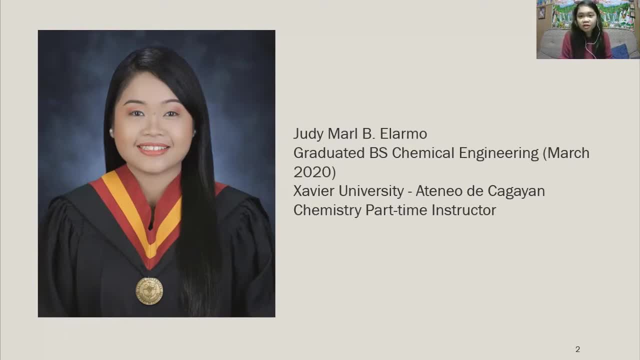 us and our other batchmates is working or is studying hard for our license, So hopefully next year. So please pray for all of us. and anyway, I'm working also right now- chemistry for an instructor in one of the most well known universities in the United States. So 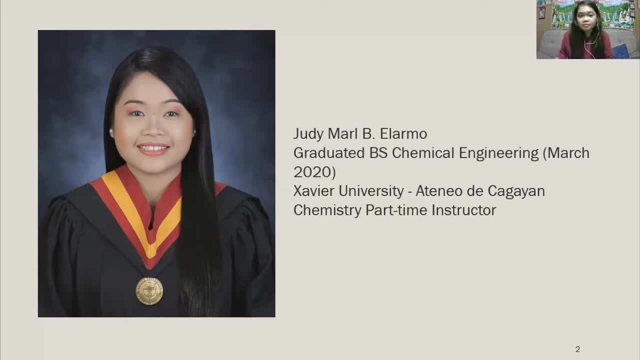 that's the reason that I came here. I'm going to be doing some research around chemistry university here in the city, So I guess that's it. I don't have anything to say about myself anymore, So if you want to reach out to me, you just have to email me. I will give you. 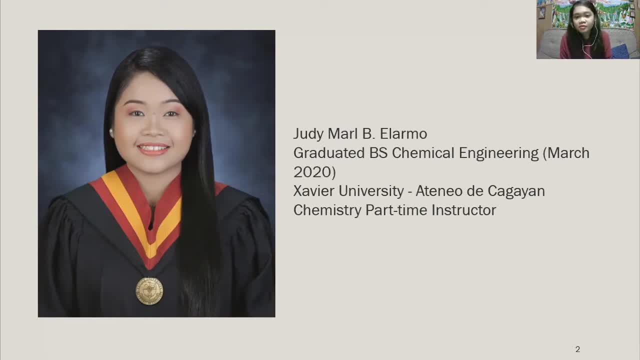 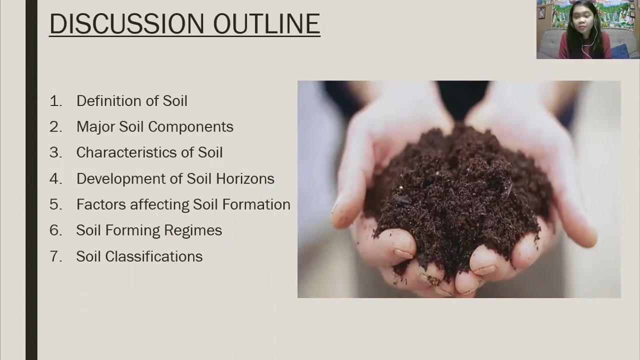 my email and then reach me out on Facebook. So my name is stated there. I'm Judy Mar-Alamo on Facebook. So without further ado, let's get started and I'll be back soon. So for our discussion outline today, I will be going to discuss seven major topics under 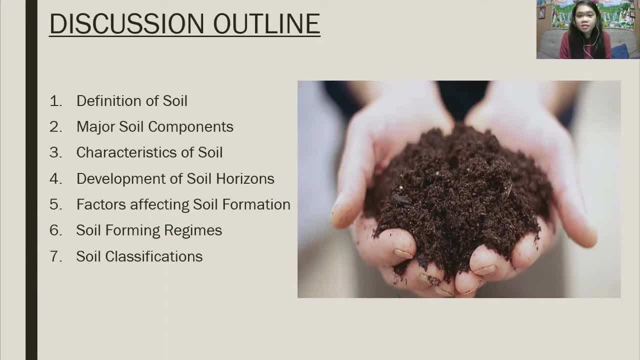 this soil chemistry. So the first is the definition of soil, Second is natural soil components, And then the different characteristics of soils, the developmental soil horizons, as well as the factors that could affect the soil formation, And then the different soil forming regions, And then the different classifications. 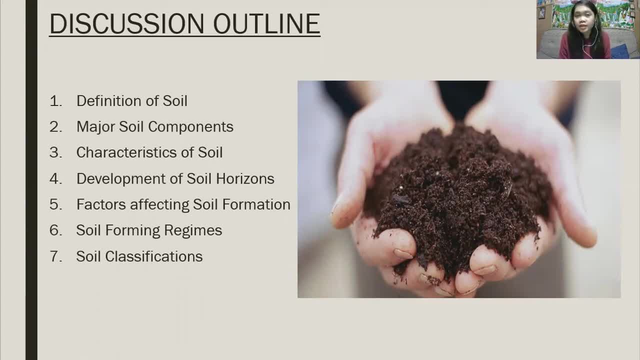 of soil. So throughout this discussion I hope that you will understand more about the soil composition here. on the topic, And as I read your lecture notes, I find it very, very interesting to learn. And then it includes a lot of ah, new terms, But hopefully, as 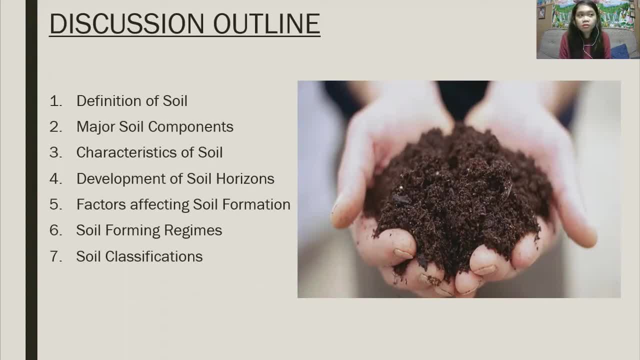 we go along, we would be able to remember those terms and it's really applicable. It's really applicable to further understanding and just to be able to transform soil settings and climate change, if you want to, to go through the next lectures. so i hope you understand. 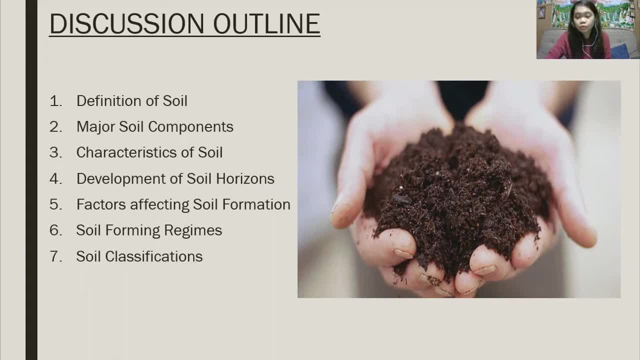 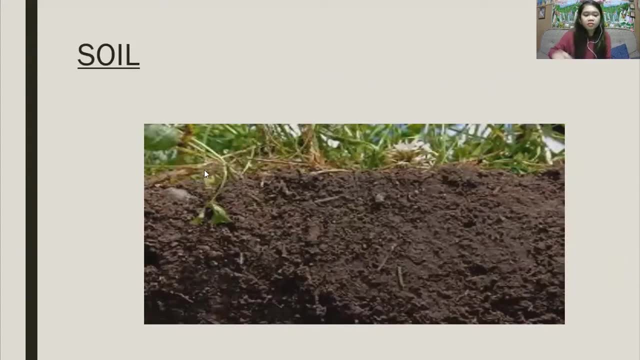 the different major terms first, before you go through so. so here we have a definition of soil, so you can see in the picture. it's really familiar for us. we know or we have seen soil. we have seen soil in our lives, so it's one of the most important. 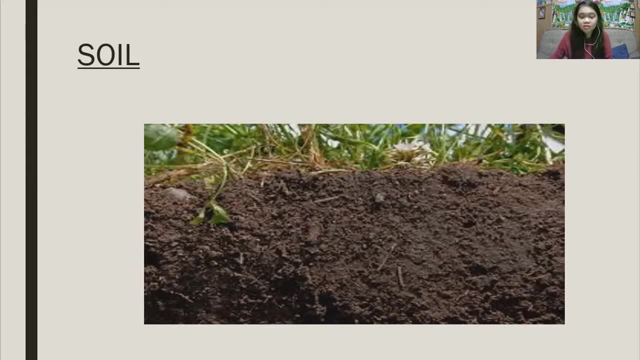 natural resource that is essential for resisting the earth's environment. so, as the definition here soil, it is the constant unconsolidated cover on the surface of the earth. it is composed primary, primarily, of decomposed rock materials and varying amounts of water gases and organic materials, and it covers 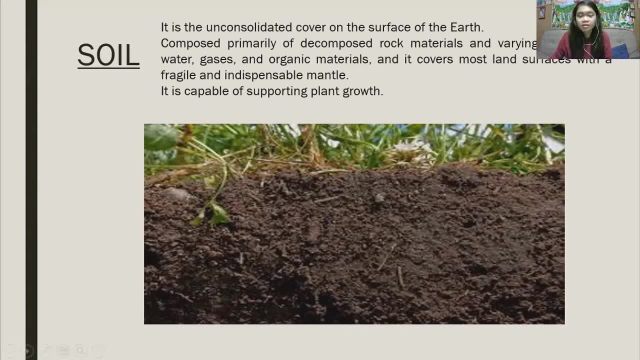 most land surfaces with a fragile and indistinct dispensable material. it is also capable of supporting plant growth. so soil, it has also been called the skin of the earth, and its condition and nature usually reflect on the environment under which it is formed and exists today. so 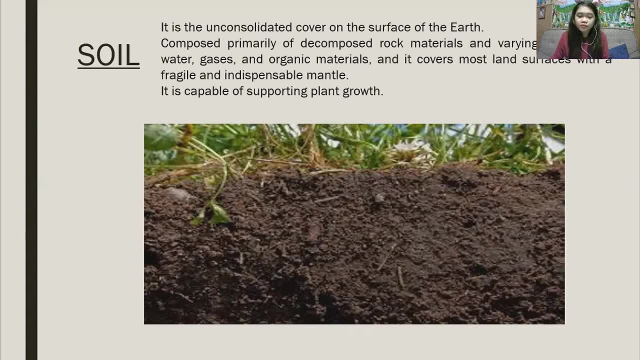 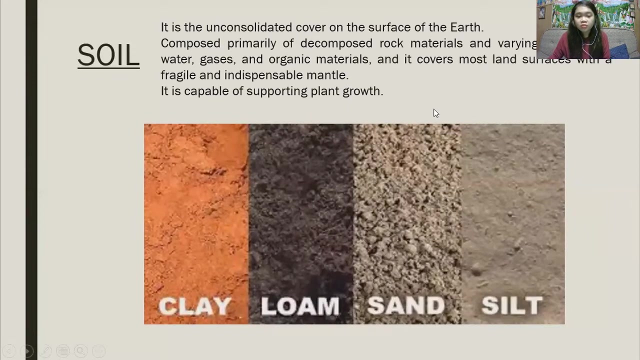 also, soil responds to different climatic conditions, especially to temperature and moisture, and to the land surface, to the land surface configuration itself, and then then to the vegetative cover, on the different types of plants and its composition into the microorganisms or animal activity. so throughout our discussion i'll be discussing four types of soil. so um. 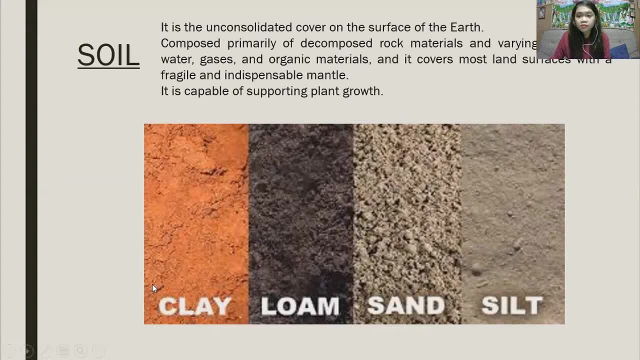 here but along our discussion, um, just be familiar that, um, the i'll be, i'll be discussing uh, clay, loam, sand and silk. so if i ever mention this in our discussion, i hope that, um, i would define, i could define them, and then and then by the uh, physical appearance, um, 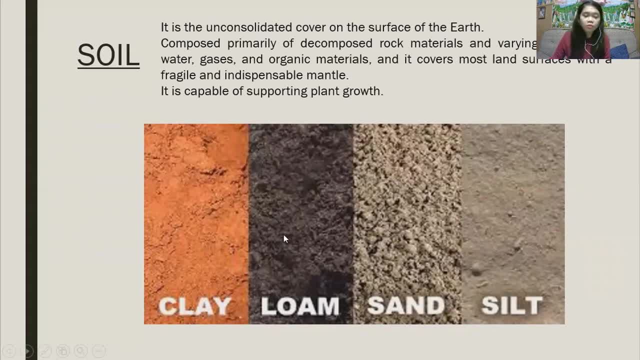 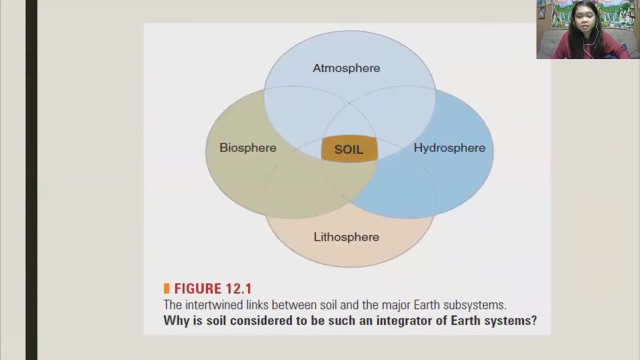 we would have an idea, uh, what clay is, what loam is in the sand and silk. so i think the most familiar that you know is sand. so so, yes, let's continue so here. um, because soil, it develops in response to its environment and with its different characteristics. 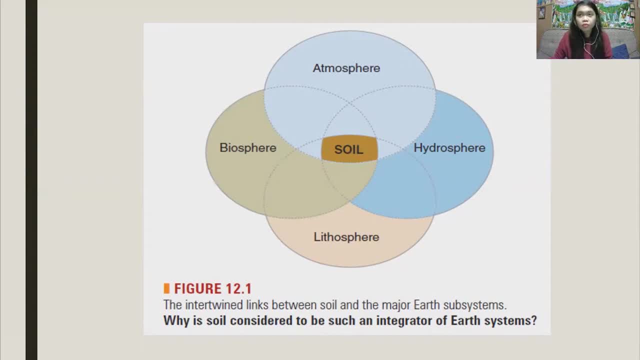 and its conditions under with uh under which it is formed. so soil is an exceptional example of integration and it overlaps among earth systems. so what i'm talking here- the different systems- is that the atmosphere, the biosphere, the lithosphere and then the uh hydrosphere. 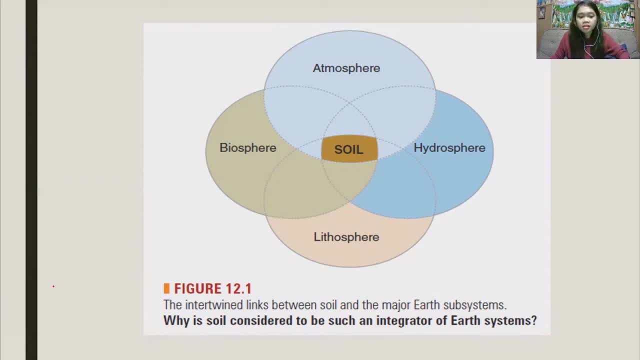 so this is an integrated system, but it can be divided into four main products, as you can see, uh, soil is between among them. uh, before i will discuss, uh, why soil is connected with this four earth subsystem, i just want to to, i just want to introduce to you this base four, so this lithosphere. 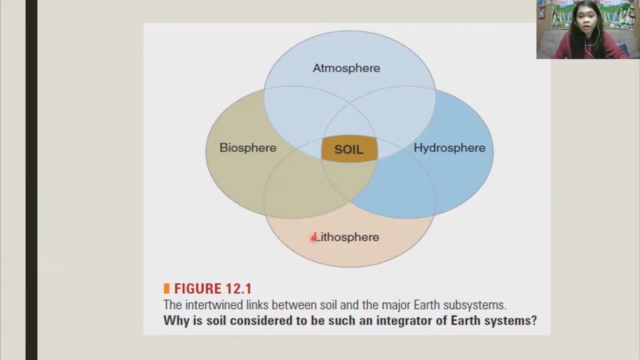 actually, this is the part of the planet that is composed of of rocks and minerals, so it includes the solid crust, the molten mantle and the liquid in the solid parts of the air score. so so usually in many places the geosphere develops a layer of soil here, in which nutrients become available to. 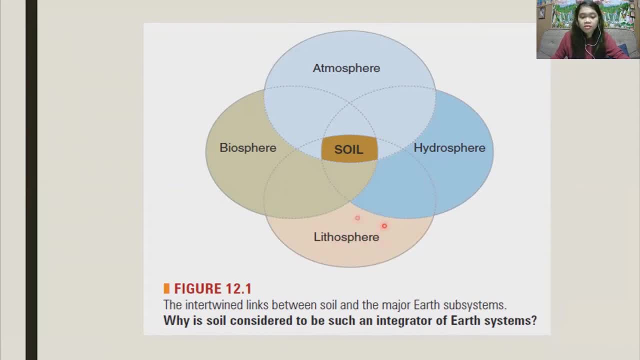 living organisms, and then um, it provides an important ecological habitat and the there are different pieces of many forms of life here. second, here is the atmosphere. so the atmosphere, this is the gaseous layer surrounding the earth and it helps its surface by gravity. so the atmosphere here also absorbs water, usually from the earth's surface, and 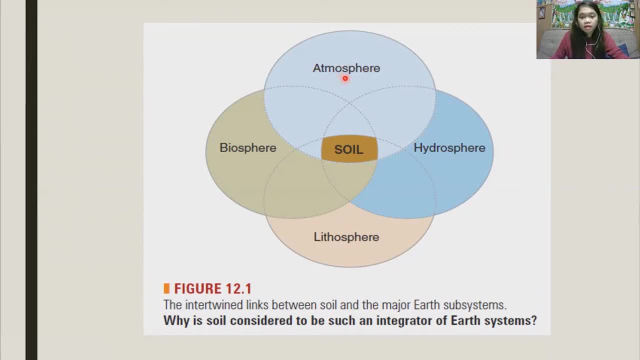 then it acts to re-distribute the heat and moisture across the earth's surface. for the hydrosphere, usually it consists of those parts of the earth system, uh, in its liquid form, so, uh, it could be gaseous or solid, the ice, the hydrosphere includes the earth's oceans and seas. 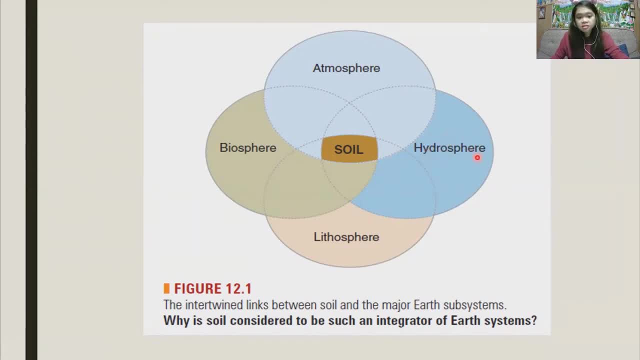 and ice sheets and the atmosphere of the earth's surface. so the atmosphere of the earth's surface, the sea, ice and glaciers and lakes, rivers, streams- this includes both salt water and freshwater systems also- and uh, the moisture, especially the moisture found in the soil or soil, water and within rocks. for the biosphere, it contains all living organisms and it is. 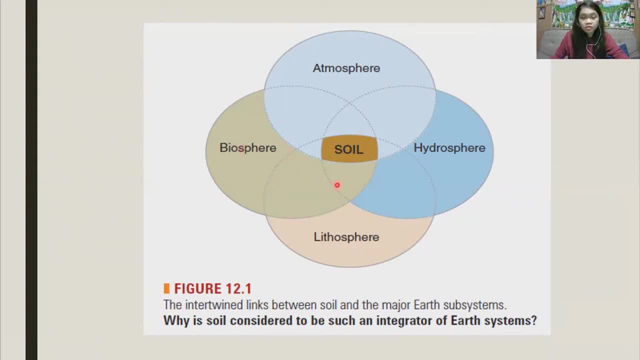 intimately related to the other three spheres here. uh, most living organisms require the issues. i mean require gases from the atmosphere, water from the hydrosphere and then the nutrients and minerals from the biosphere. so the question now is that, um, what is actually uh soil made of, and what does this the? 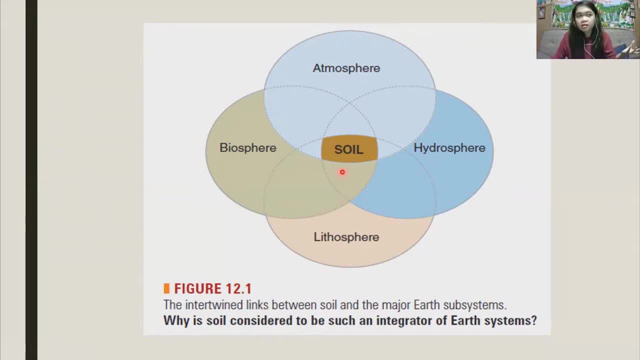 if you imagine, if you scoop a certain, uh, certain amount of soil using a shovel, what are these, uh, what are these uh, soil compost from? so, uh, uh, for the next slide, i will discuss to you the the uh soil function. soil function as, as a open system. so you imagine, uh, there are. 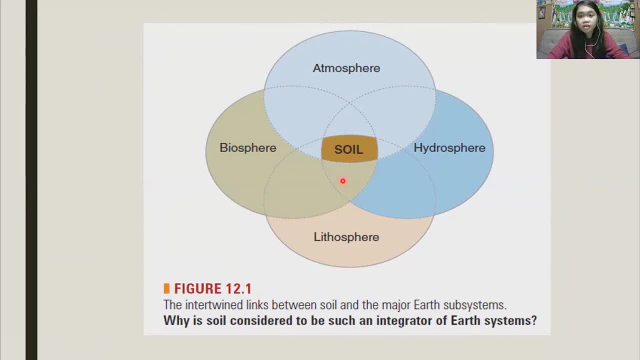 open system. you have open system, right. so there are matter and energy that flows in and out of the soil and they- some are also held up in storage. so if you understand, this flows uh the input and the output, so the components and processes uh also involve. you could also uh be familiar with it. so 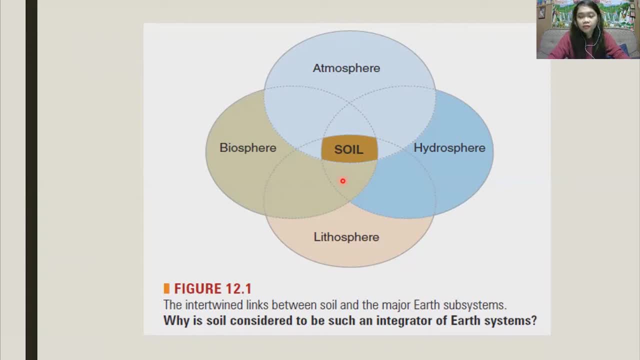 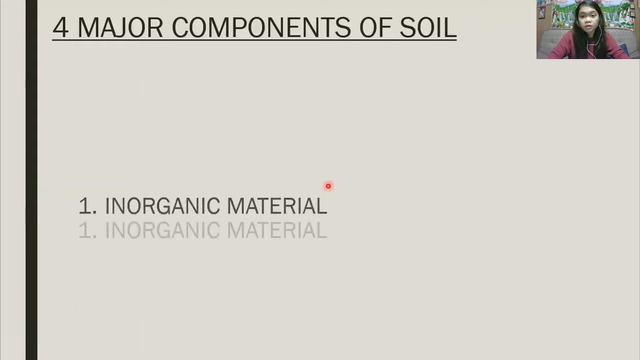 so that's very, very actually vary from uh soil to soil. so uh, you have to to appreciate or to understand its complexities and its critical natural resources and its function to the environment. so here we will discuss the four components of soil, mainly in organic material, soil, water. 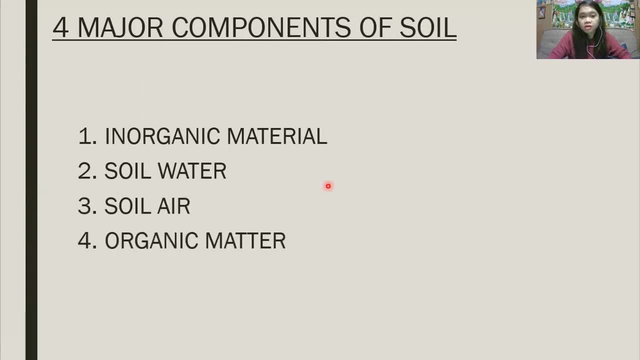 so soil, air and organic matter. so these are the four major components of the soil. so from a study, so from a study study, uh, 25 percent of the components of soil are usually uh, is air, and then um, 55 percent food is water, and then for mineral, mineral material, or you know, these are inorganic materials. so 45, 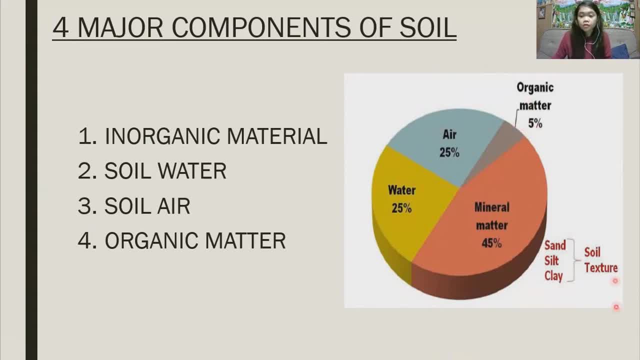 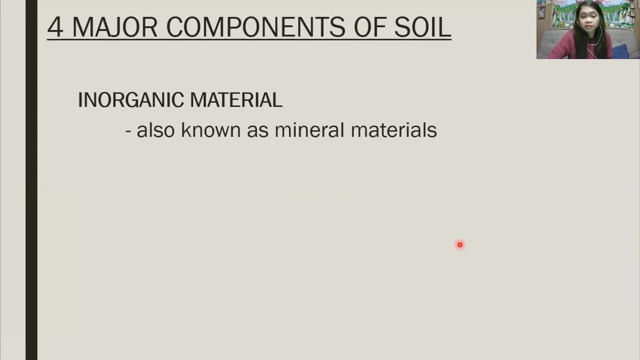 and then um five percent long organic matter. so, uh, the further slides, or the next slides, i will discuss this for. so we'll go start with inorganic materials. so it's also known as mineral matters, and in mineral materials this uh includes soluble minerals found in soils that are combination of 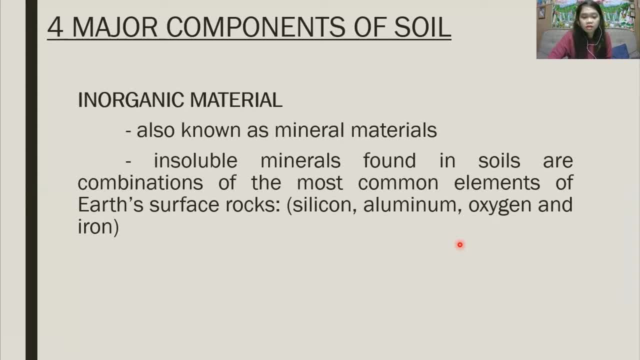 the most common elements of earth's surface, such as silicon, aluminum, oxygen and urine. so, if you say in soluble minerals, these are constituents that occur, a solid compound so, and it can't be dissolved in water. and some of these insoluble minerals are usually found in air or water that are essential for the components of soil. so 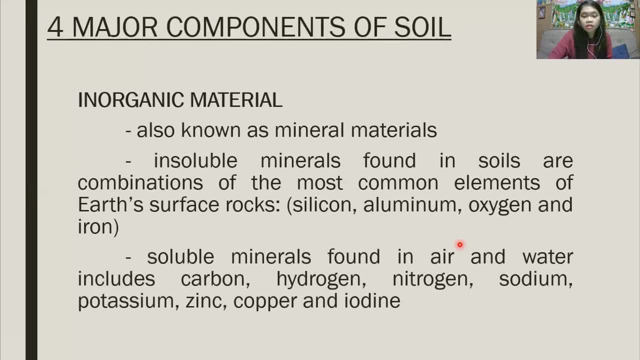 we have also soluble minerals found in air and water, which includes carbon hydrogen, nitrogen, sodium, potassium, zinc, copper and iodine. so this inorganic material, usually they are the ones that sustain the soil deficiencies for specific plants. soil deficiency: here is something that uh, uh, that, uh, certain matter that soil lacks. so 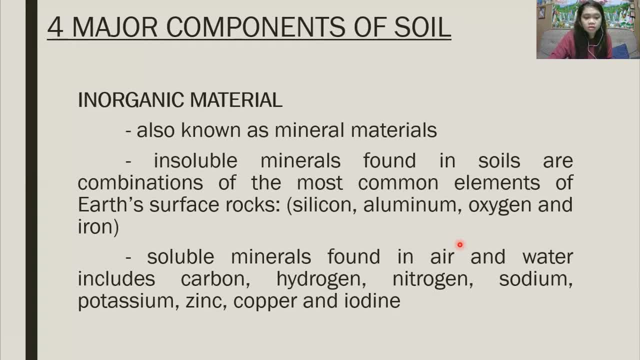 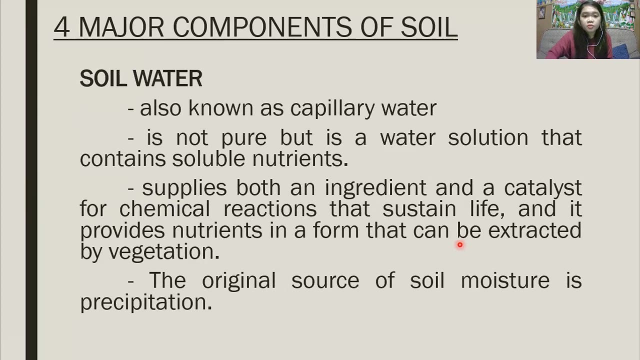 uh, introducing them. the process of soil fertilization: this is the process of adding certain nutrients or other constituents to the soil in order to meet the conditions that certain plants require. so the addition of of of these certain nutrients are usually in organic material. so so also we have uh soil water. so soil water um. 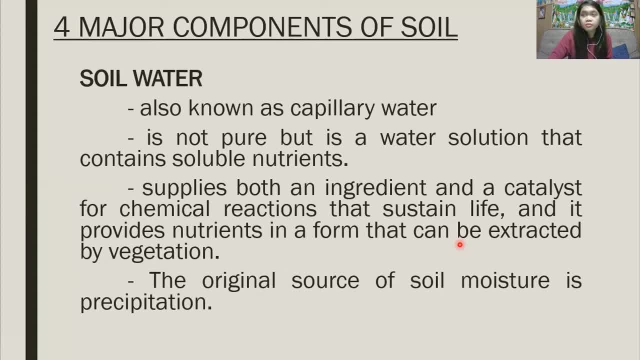 it is also known as capillary water. so we will be mentioning capillary water often in this presentation. so if i mentioned that, it usually talks to soil water. so it is not pure but it is a water solution that contains soluble nutrients. so the function of soil water: it 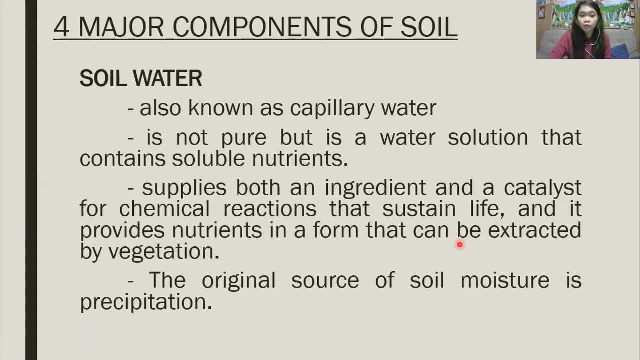 serves uh as a stored water supply for plants, and it also supplies both as an ingredient and- i can't- a catalyst for chemical reactions that sustain life, and it provides nutrients in a form that can be extracted by vegetation and and the original source for soil moisture is precipitation. so 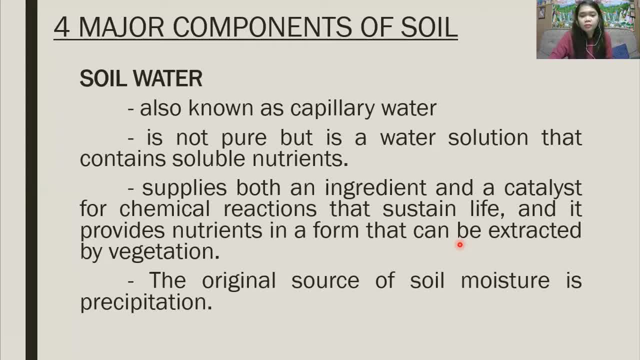 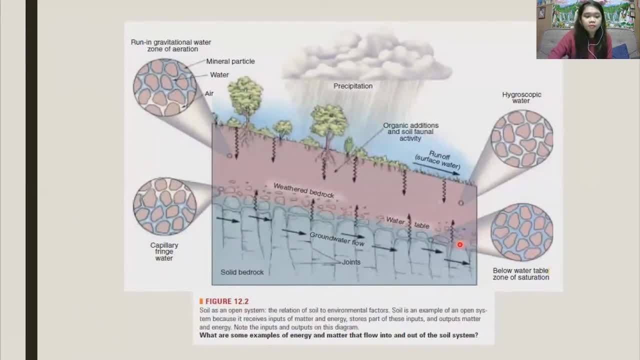 uh, the what, uh, what. precipitation is actually a process. so here precipitation happens when, as a rain, there is a rain and then it falls on the land. most of it is either absorbed on the ground or run, or it runs along the, along the soil or down slope. so what they're? 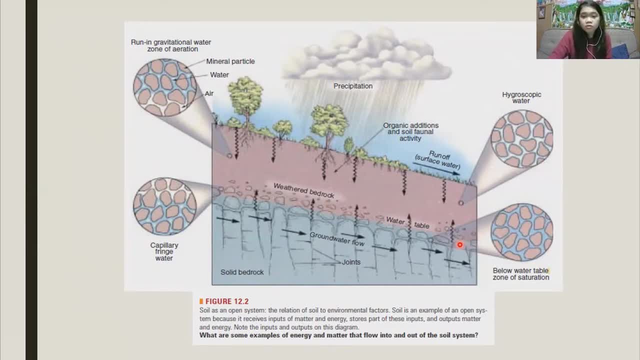 seeing through the soil, washes over and through various soil materials and and by doing so, it dissolves some of these materials and carrying them through the soil. so basically, um, we have also this uh concept called uh, soil gravitational water. so this is the, the one that i'm talking about. it is the, the amount of water flowing down, the 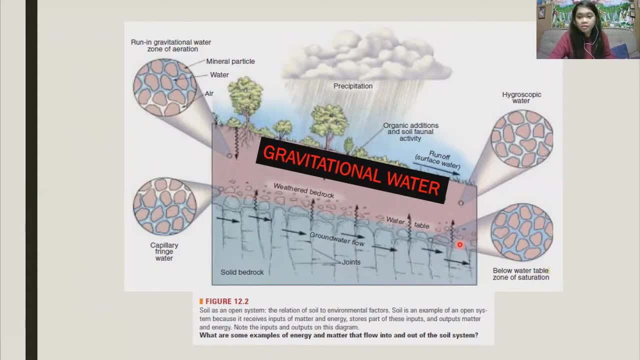 down slope as rain, as rain happens. so let's look at this figure to see where the water in the soil is found. uh, in several different circumstances. so what they're here it comes, uh, it goes down to the soil, it goes down through the soil and under the force of gravity, so we have this gravitational water. it moves downward through the 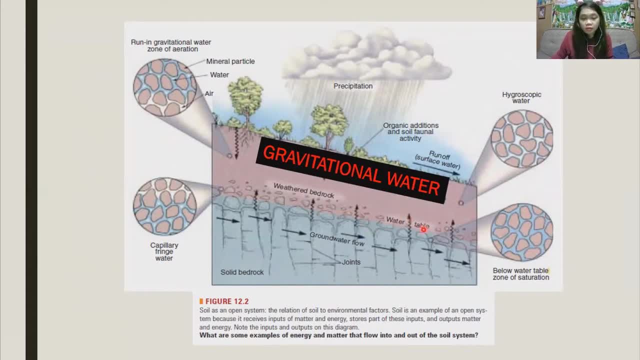 soil particles uh towards this uh water table here, so doing so? uh. actually, this water table here is the level below uh, which all available places in the rocks and soil are filled with water. so, as a consequence, water cannot go deeper. so the quantity of this gravitational water in the soil 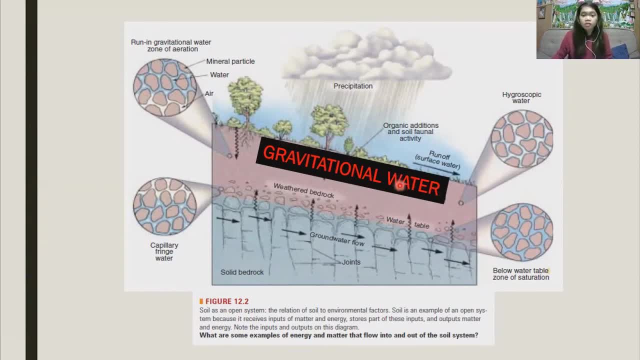 is related to its real conditions, so it includes the amount of into the soil internal water found of precipitation and the time since it fell. so so, because, um, because, as uh, the longer time it goes to the soil, some of these will evaporate. and and it also take into account how easily the water 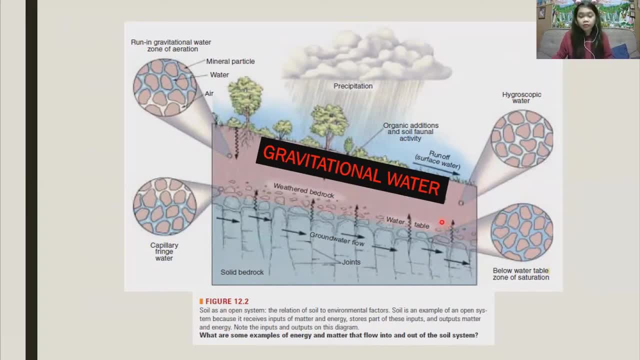 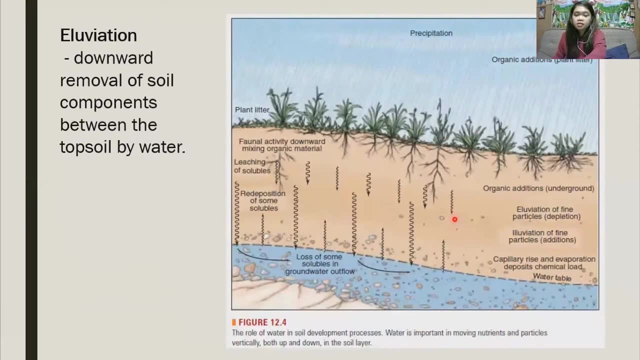 can move through the soil and the space, has a real point for water storage. so now let's see, now let's see, um, how this gravitational water functions in the soil in several ways, through this figure. so first, uh, gravitational water, uh, it moves down to the soil, takes up. 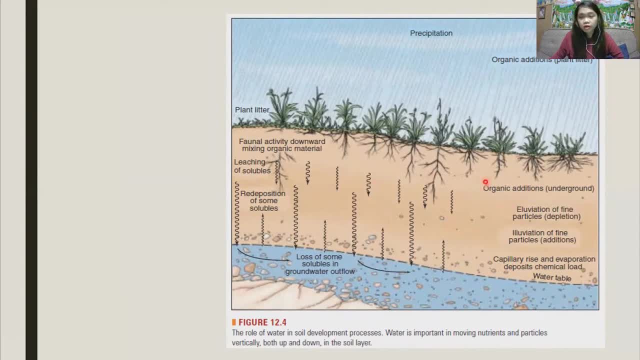 and it picks up with finer particles for, as i as i said, uh, clay or silk here. so if i say tiny particles, types of soil, which includes the clay and silk, so, uh, usually it comes from the upper layer of the soil and then this downward removal of 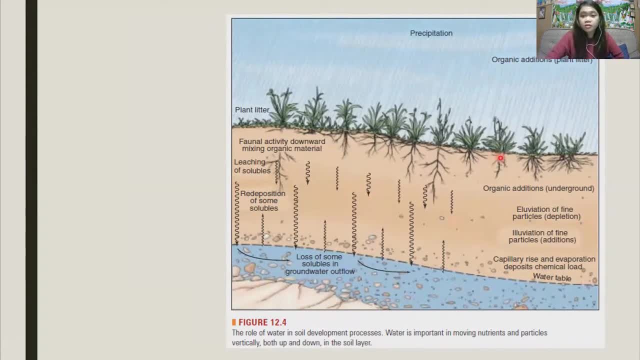 soil components from the top. soil is called the process of innovation. so this here, uh gravitational water is going down. it's moving down, uh, through the soil and it picks up those uh finite particles which are the usually the clay silk from the upper soil layers, and by doing so we have the process of innovation. and then we have 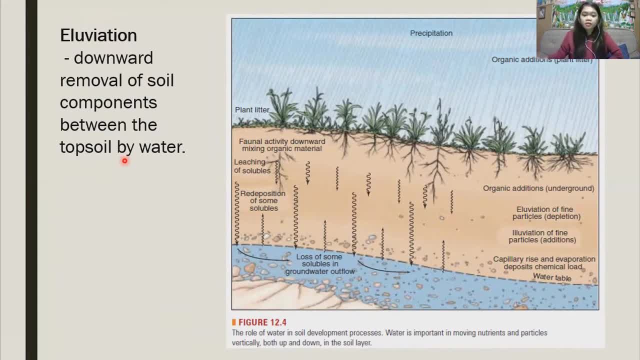 also um another process: if, uh, gravitational water continues to move downward, uh it deposits and it deposits the, the fine materials that it gets from the upper layer and, um, usually it deposits in the much more lower level of the soil. so this process of the position of fine materials by water, 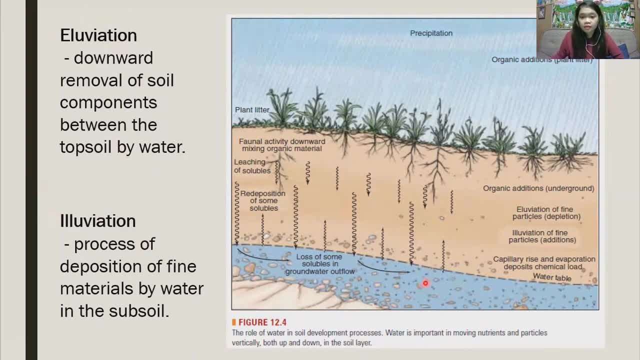 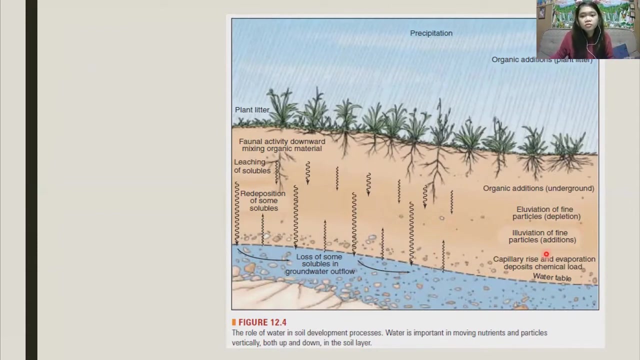 is called the process of innovation. here in this picture, we have the process of innovation below in innovation. so this is the uh, the position of fine materials from the upper part of the topsoil, so also um, as you have it here in this picture, you can see that the gravitational water continues to move downward. 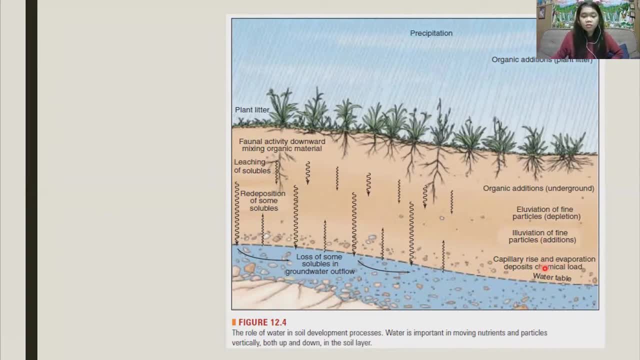 so it resolves. so you will inorganic uh, inorganic materials or minerals, and it carries them more deeper on the levels of the soil. so, um, perhaps it could be on the zone that uh, where all of these open systems are saturated and will be great with um, this uh, soluble inorganic materials. so 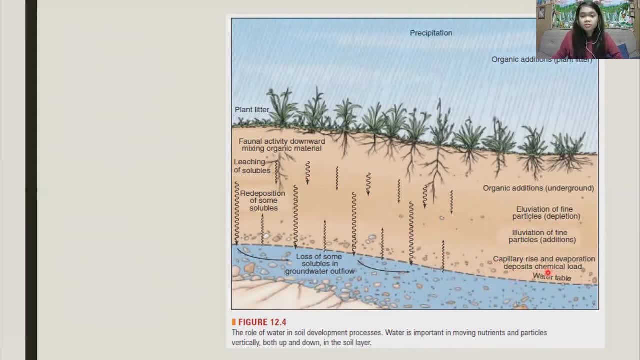 by doing so um depleting these nutrients. you will put these nutrients into the upper soil by the process of leaching, to the process of leaching using the flow of water. so leaching here is the process of depleting nutrients in the upper soil by the thorough flow of water. so so, in summary, uh. 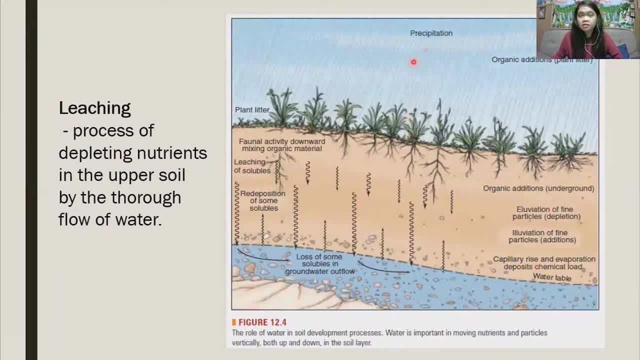 as precipitation happens, we- uh i mean the aspect which precipitation happens, gravitational water- wash out the the fine particles uh, and goes into the deep, uh part of the soil which is called elevation of fine particles. here which is the innovation. and then and then, as the gravitational water more goes, more deeper, it deposits the fine particles. 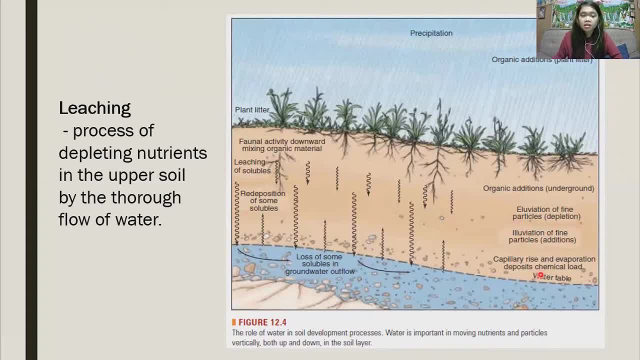 so this hot is the process of illumination. and then, um, we also, uh, we also- take into account the soluble inorganic minerals that are carried into a much more deeper levels of the soil so it deposits on, on, on saturated species along here, so by the process of a thorough flow of water. 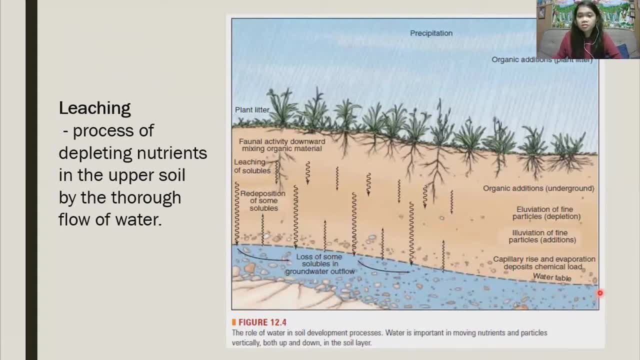 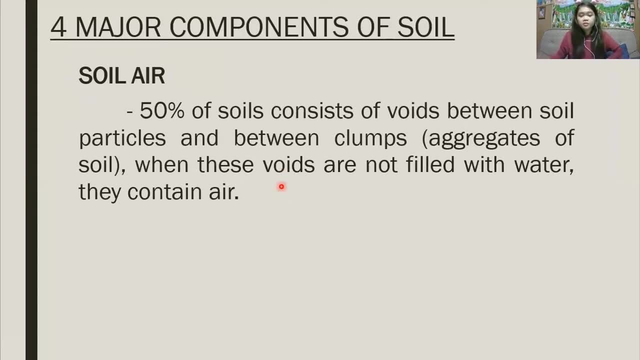 these nutrients will be distributed and the process is called leaching. so another component of soil we have, um, we have soil air. so soil air- it is 50 percent of the soil consists. uh, we know that 50 percent of soil consists of voids between soil particles and 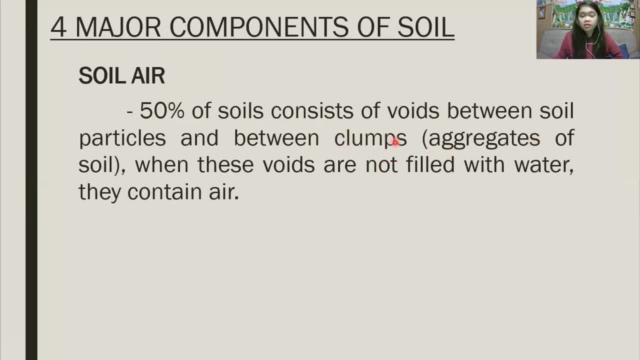 between plants. so so the plants here are the aggregates of soil and in this uh, when these voids are not filled with water, they contain a lot of water air, so it's likely to have less the air. also, it's likely to have less oxygen, more carbon dioxide and a 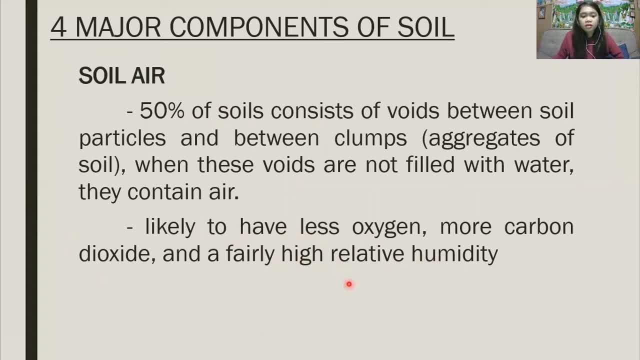 fairly high relative humidity. so so the uh compared to the composition of the lower atmosphere, the air in the soil usually um. it takes to have less oxygen and more carbon dioxide and a high relative humidity because the presence of capillary and and and or the soil water. so 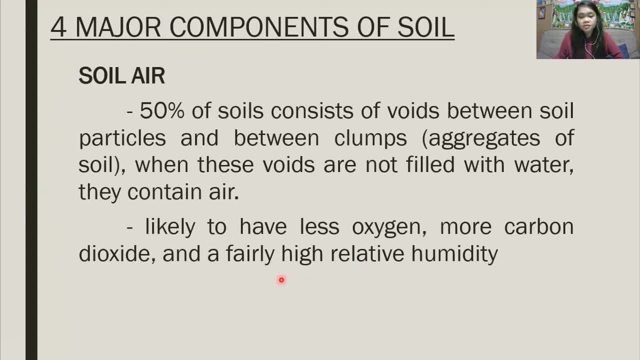 for most, or the microorganisms and plants that also lives in the ground, uh, soil, air, soil, areas that lie oxygen and carbon dioxide, necessary for them for my purposes. so it's also a very big. they can help for those microorganisms living, living in the. And then the problem of water: saturated soil. they are not necessarily excess water, but if all pores of the species of the rock is filled with water, there is no air that can go in. 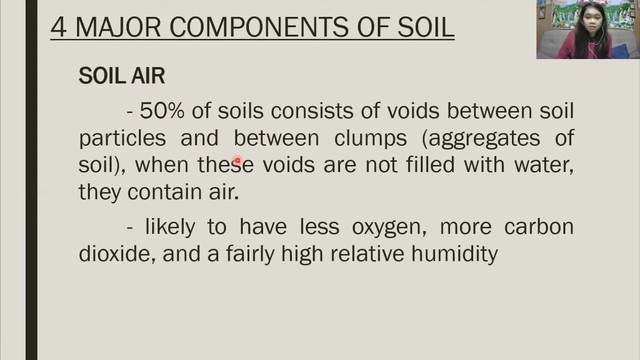 So the lack of air is why many plants and animals find it difficult to survive in water-saturated soil. So it's very important that those voids of the soil must be contained with air to help those microorganisms also leave the ground. So 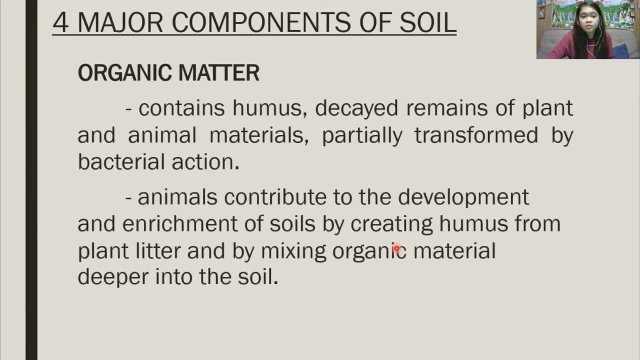 For these, The last component or major component of soils, we have organic matter. So this organic matter contains humus. These are the decayed remains of plants and animals, animal materials partially transformed by bacterial action. So humus actually is an important part of plant growth or vegetation process because it acts as a catalyst. 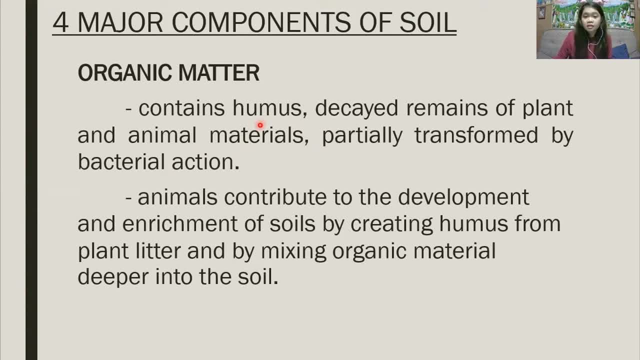 Usually in chemical reaction, by which plants here extract soil nutrients and minerals that it provides to the soil. So a soil that contains humus is quite workable and has a good capacity to retain water. It also provides food food source for microscopic soil organisms. An example here could be bacteria. So, for example, here we have a plant that contains humus. So, for example, here we have a plant that contains humus. So, for example, here we have a plant that contains humus. 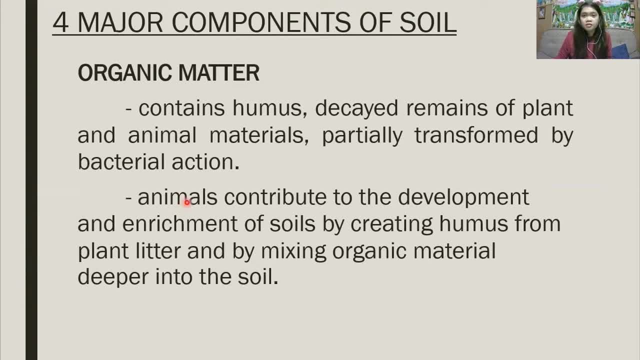 Also the interes of the soil it contains. It contains mucosi and aniline as well. It contains bacteria and fungi, up to the earthworms and many other microorganisms found in soil. Also organic matter. Animals contribute to the development and enrichment of soils by creating humus for plants deeper and by mixing organic. 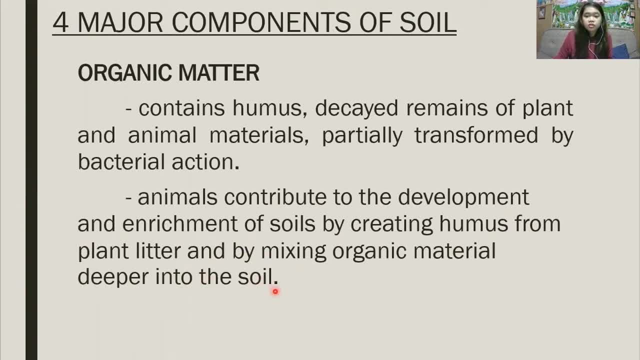 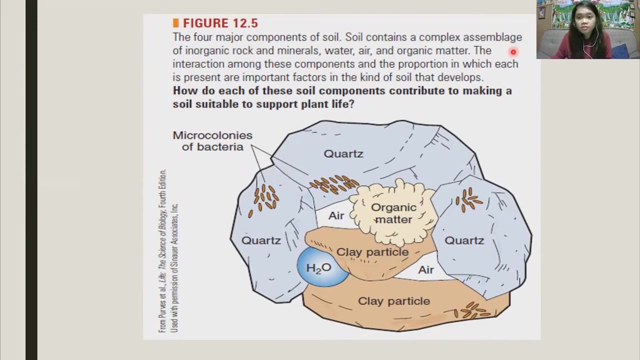 materials deeper into the soil. In addition, chemical and mechanical functions of plants and their root systems are usually likeassembled, integral part of soil farming system. so they use mostly organic matter to sustain the nutrients that they need in order for them to grow. so this is the diagram for the four major components of 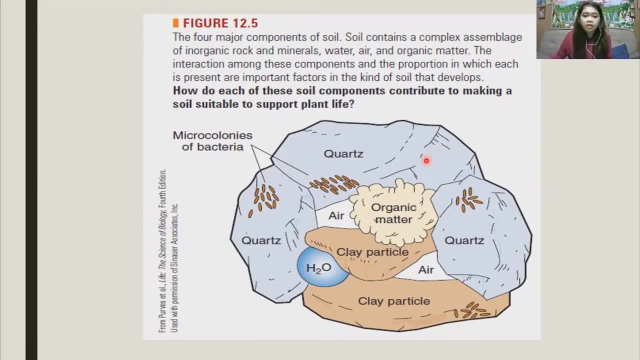 soil. so i've mentioned here that these are the- uh, we have here the inorganic material- inorganic materials, so it's mostly on the outer layer, and then we have found here the soil water. so we have here the water and then we have the organic matter. so i think this is the humus, that that is discussed. 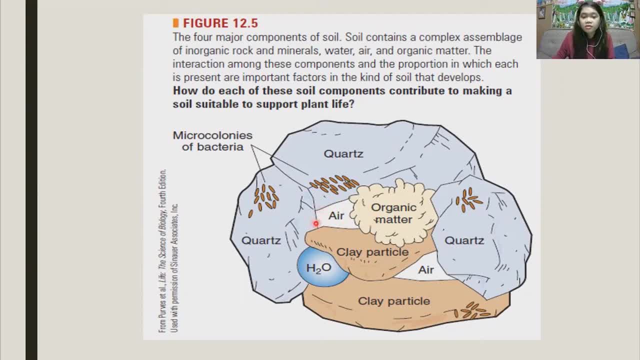 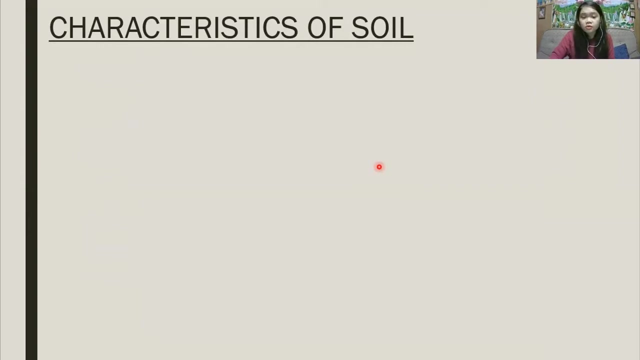 in the uh past slide and the voids here they are composed of air. so this is the uh. this is the diagram or picture for the major components of soil and its designation. now we go to the different characteristics of soil. so soil, soil properties can be readily tested and examined. 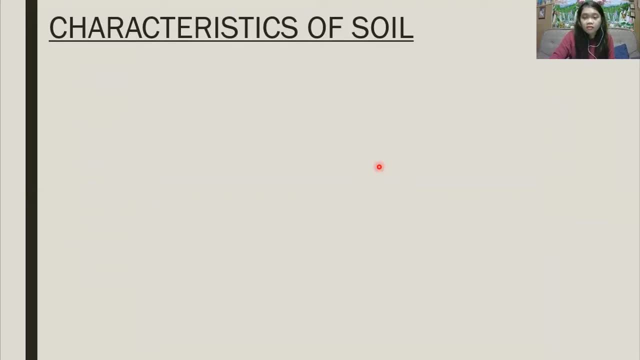 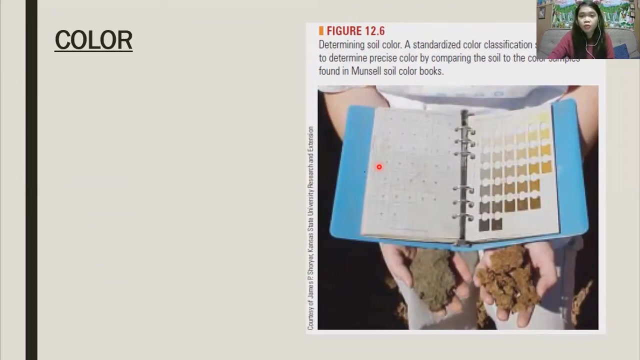 and the hours they are being used to describe different soil types. so so the first is that we have color, texture, structure and acidity or alkalinity. so i'll be discussing these four also. let's start with color. so most people, actually we, are aware that soils vary in color. 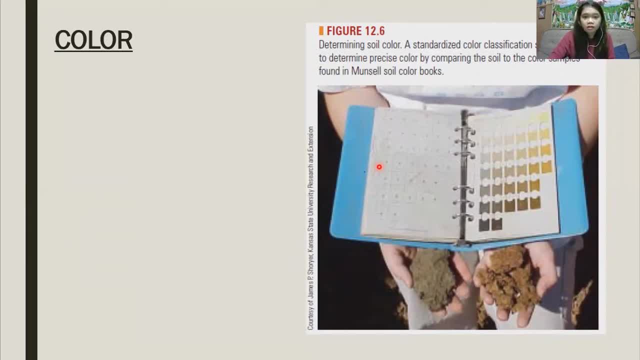 or from place to place right. so, uh, usually color: this is the most visible attribute of soil: very, very physical and very visible. okay, usually this is the first one that we see, and then it vary in color, usually from black to brown to red, yellow, gray and near white. so 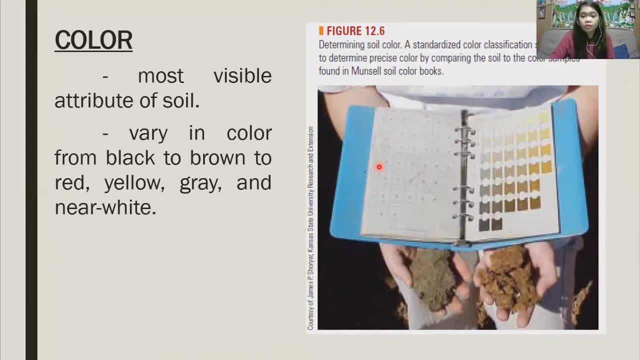 so later i'll be discussing what. what composition does uh soil had if this is this color? i mean, this is the color and and what does it? it contains. so also a soil scholar offers a clue to its physical and chemical characteristics. so in this picture this is uh, uh called the moncell color book. 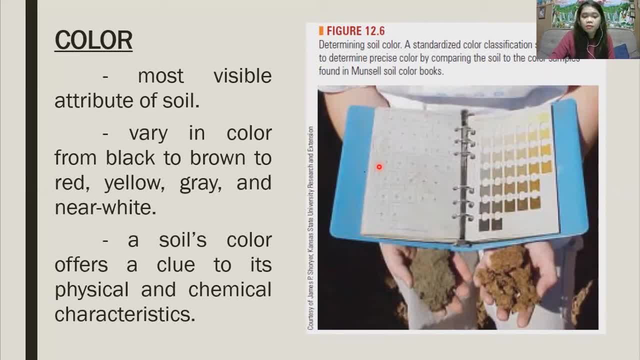 this is the color book that is usually used by laboratory soil scientists when they want to describe soils in the field or samples that they collected. and then this is a standardized soil color book- and usually it is. it is used to identify what type of what type of soil have they. 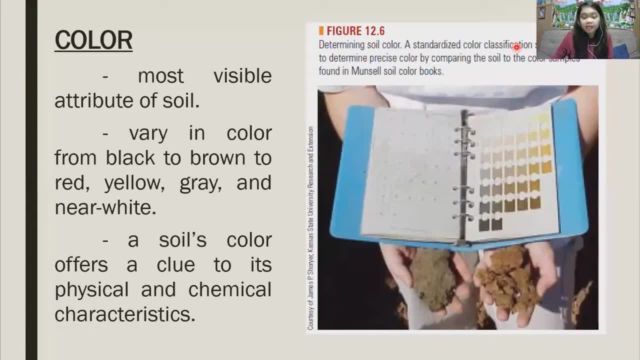 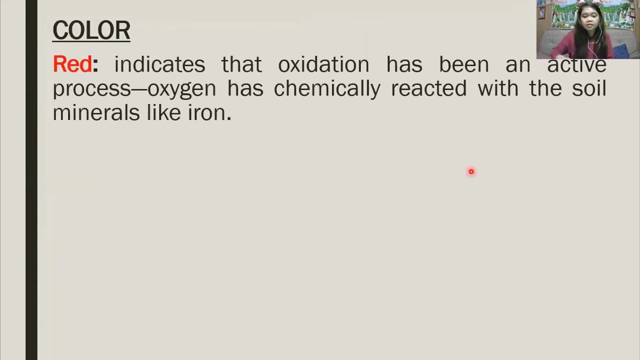 collected. so it's a standard guide, usually for matching and recognizing precise color of soil types, and this book also includes common soil colors, colors or colors, but each color can also appear in a wide variety of tones here. if that um, um, if you collected, for example, if 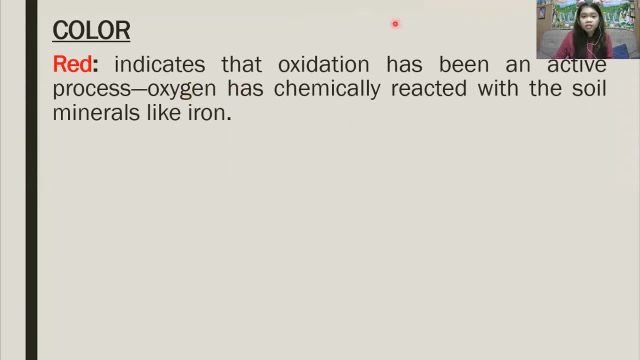 you collected a soil that is color red, usually it indicates that oxidation has been an active process here and oxygen has chemically reacted with the soil minerals like iron. so so, um, if you you see a red color soil, usually it contains- um, it contains iron, iron minerals and and oxidation. 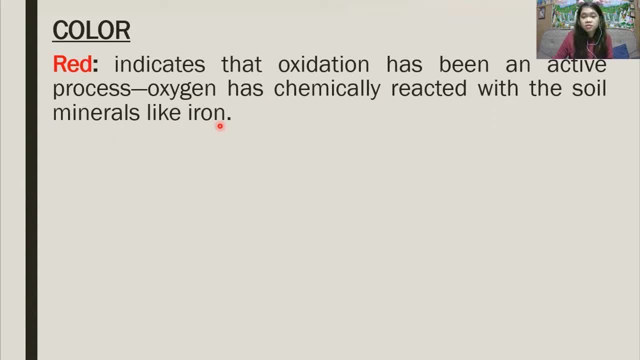 happens, it reacts with oxygen. so if you collected a soil that is color red, you can see that it has a reddish color. so for blue, silver and gray, usually these stones mean that the soil has been, the soil has likely been reduced, in other words, oxygen has been removed from the soil. so 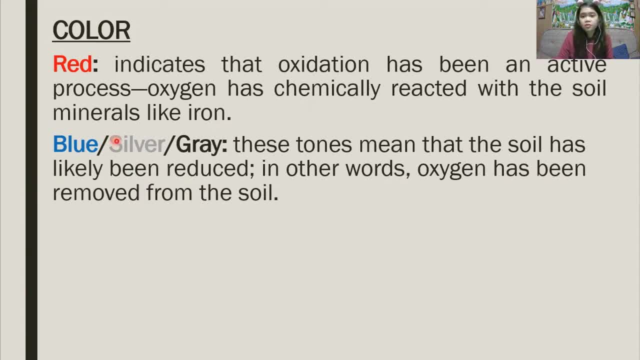 even if, um, even if this type of soil also consists- it says um iron minerals- then, um, it does not, uh, react with the oxygen on air, so, so, um, it has less oxygen content. that's why the color here, instead of red, it becomes blue, silver or either gray. 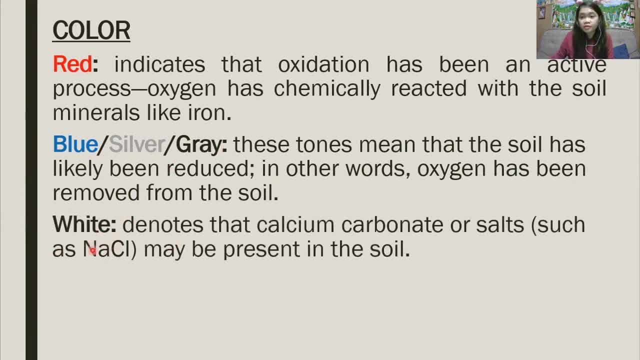 you have also white. um, i did not color it white because you could not see the word, so, but i know what you're. you know the color white. so usually it denotes that calcium carbonate or salts such as sodium chloride may be present in the soil. so if you see this type of soil color, 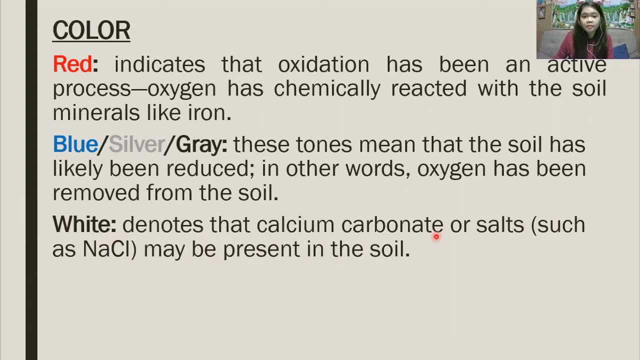 then it denotes that salts are present and then if you have also black, so a very dark color, may indicate a high amount of organic material present in the soil. so basically, black color usually here at the lugar, and then people, as what i've observed, um, uh, most of the plants, uh. 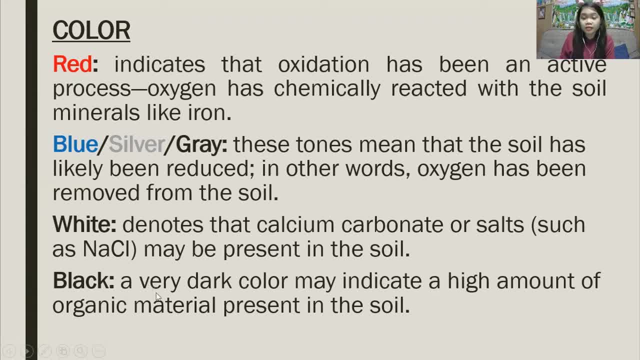 planters or farmers. they use um black, a very dark color uh soil. they know that it contains uh- most of the minerals and nutrients and organic material that uh is used for. that is good for the plants and they use this as a way to help them to uh, to help them grow the plants that they want to. 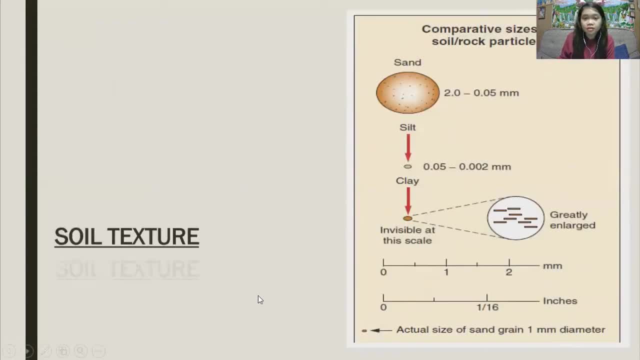 that they want to grow or plant. so now we go to another characteristic of soil. this is called the soil texture. so perfect texture. they refer to the size or distribution or sizes of particles that make up a soil. so In this picture or diagram we could see that mostly in plain type of soil. so here the 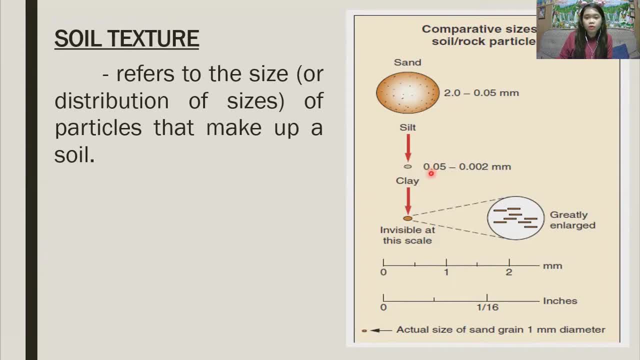 diameter ranges usually from 0,. I mean for plain soil the diameter usually ranges less than 0.02 mm. so it's very small, so it's invisible at this scale. so if we enlarge this, this would be the picture. so in salty soils also, the diameter range from 0.02 mm. 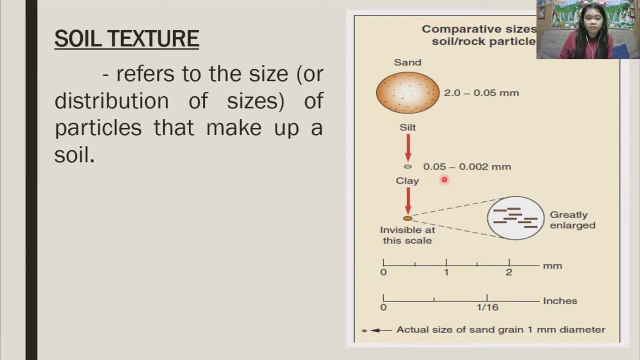 to 0.05, for sandy. these are quite big soil particles, so the diameter usually range from 0.05 to 2 mm, so particles larger than 2 mm. these are usually treated or regarded as pebbles, rocks, gravel. 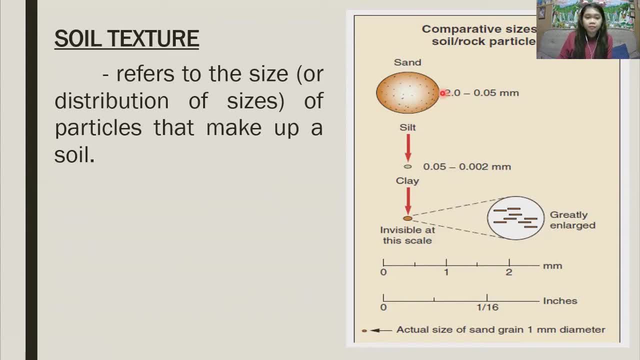 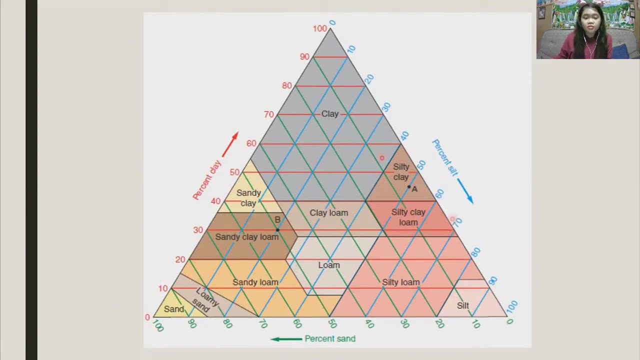 And then other types of high particles already. so here the texture of the soil also can be represented using this diagram. so we will be doing a little game here. it's a game, but it's not. You could understand that the soil is very small, so it's very small, so it's very 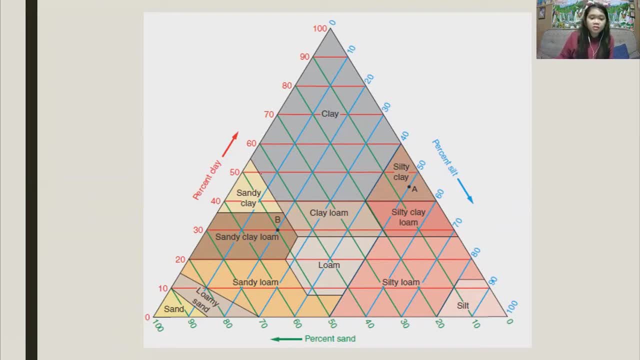 difficult to understand the soil texture using this diagram as well. so the proportion of the particles according to the size determines the soil texture. so for example here a soil composed of 50% silt-sized particles. so before we answer that we take into account. 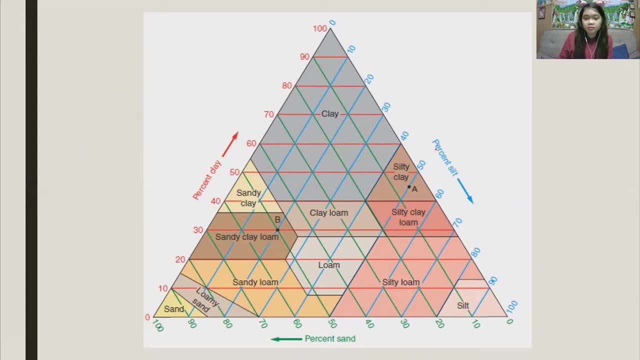 that this area. here these are the percentage for silt-sized particles, And then the red here are the percentage for percent clay. so the percentage here are from 0, increasing from 0 to 100, and then for percent soil it's from 0 to 100.. 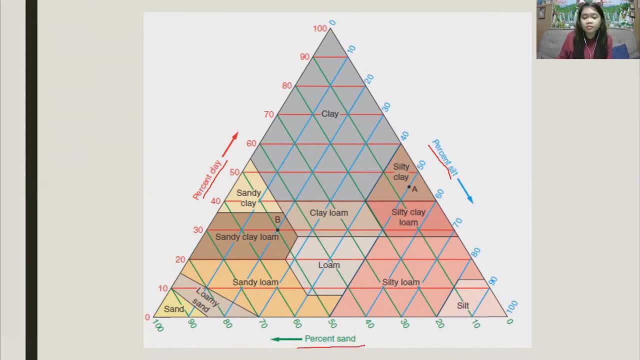 So in the bottom part we have the percent size. so for example, a soil is composed of 50% silt-sized particles And then the red. here are the percentage for percent clay. so the percentage here are from 0 to 100, and then for percent silt-sized particles. 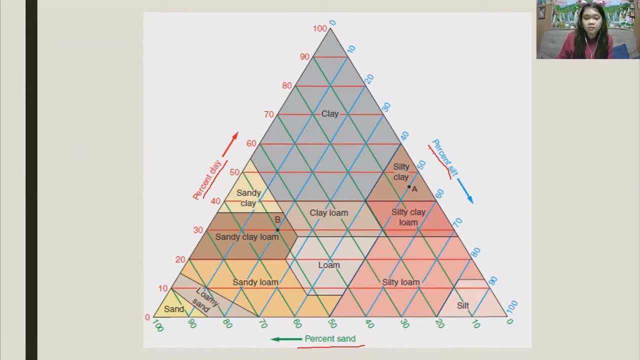 So we want to find the 50% here in the percent silt size. so this is the 50%, so we're going down, We take this part here. so we have also 45% clay. so clay, here we want to find 35%. 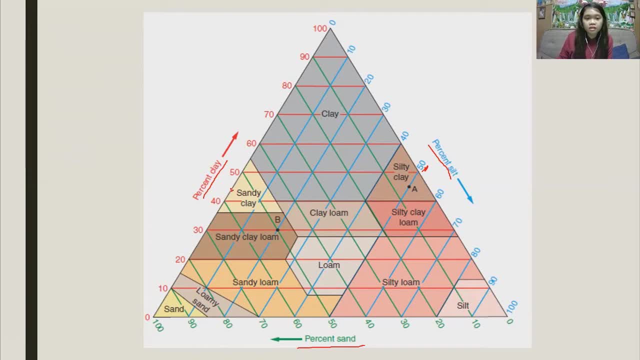 so it's between here. so we take into account this area, these two, Okay. And then it also contains the 5% sand, so here we want to find 5%, so here, 5%, Okay. so what you're going to do is that you would be identifying what type of soil is. 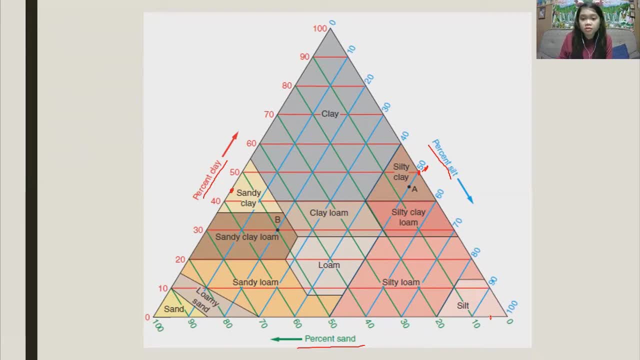 given or described, based on the percentage We go this up to go upward. Sorry, I have a very crooked line. We go upward and then we also take this horizontally, So you could see that the three lines intersect here. So it's a silty type of soil. 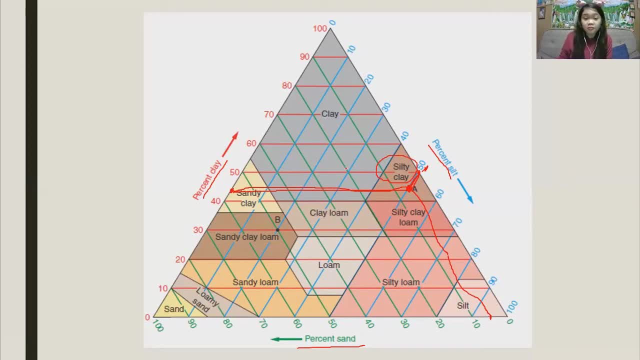 So we have described here the soil texture based on its quality. So it's a silty type of soil texture based on its composition. So here Example. another example is that a second soil sample that was given 20% silt, 20% silt. 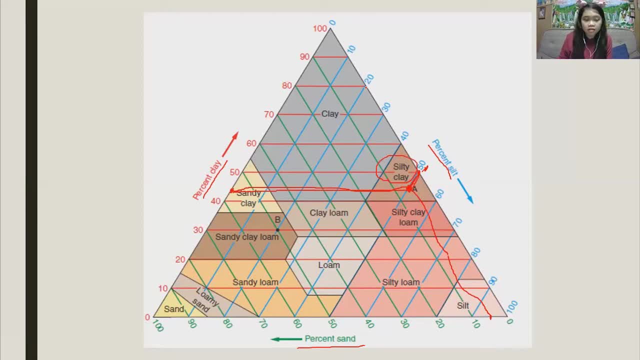 so here And then 30% clay, 30% clay, sorry, here 30% clay and then 50% sand. so we would identify what type of soil here. So we're doing the same thing that we did. 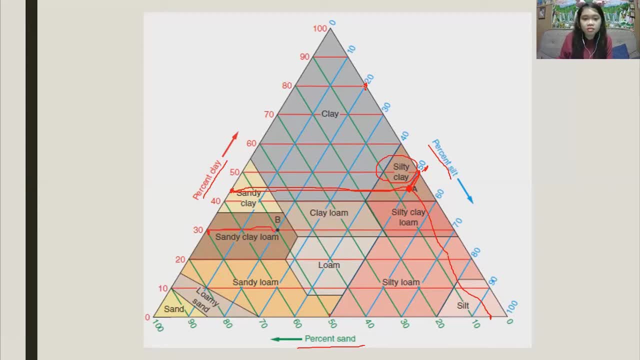 So we have identified the .3 here. So this is the sandy clay loam type of soil. So now, now I have a question for you, So you could answer this in your free time: What would be the soil type if it contains 40% sand, 40% silt and 20% clay? 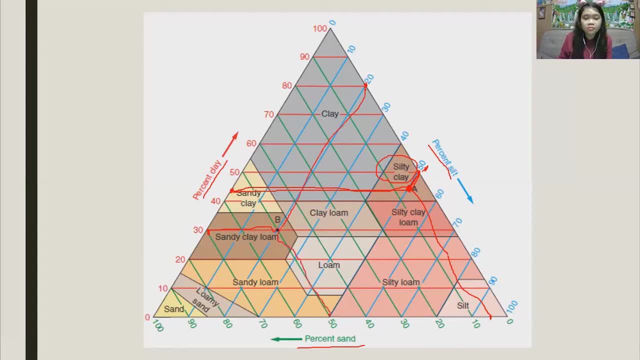 So you can answer this in your free time. So what would be the soil type if it contains 40% sand, 40% silt and 20% clay? Okay, So you can use this. Okay, So can you? can you give a quick explanation? 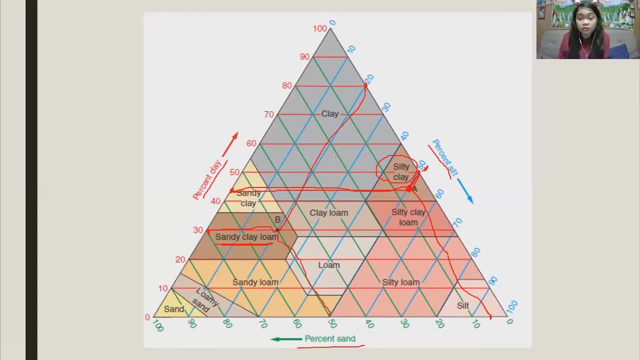 So it's not a soil type. It's a soil type. it's not a clay type. It contains 30%. it contains 30% silt, 40% and 20% clay in your free time. so what would be the soil type if it contains 40 percent sand, 40 percent silt and 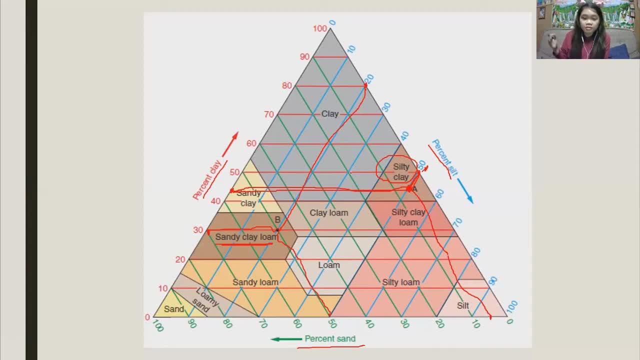 20 percent clay. so again 40 percent sand, 40 percent silt and 20 percent clay. so you can tell me, uh, what the answer is. so, uh, you could answer it now. so, okay, i just give, uh, maybe five seconds, five, four, three, two, one. 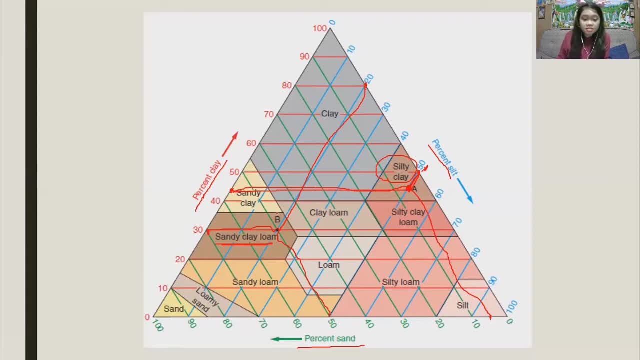 i guess, okay, okay. so the answer is, uh, if we have uh 40 percent sand, 40 percent, 40 percent silt and 20 percent clay, so what we get is a loam. so here we'll be defining what long soil is. so long soil, this type of soil? 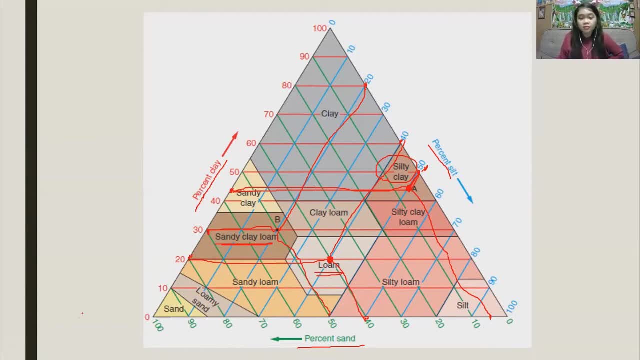 usually, as you can see, most of those types are indeed between this triangular diagram and those- uh, none either other other sides. it's the other type of soil already. so this long soil is very, very best suited for supporting vegetation growth. so i guess we already understand it. 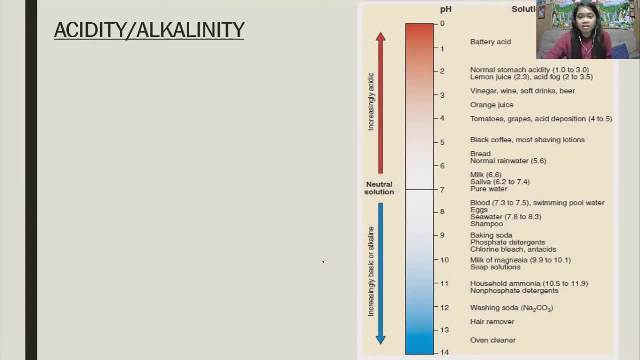 now we go to another characteristic, which is the acidity or alkalinity. so so, acidity or alkalinity, it tells if the soil is fertile or infertile, and then, um, it means that, um, uh, there are different chemical processes that takes place in most, most soils and plant systems that could make this soil fertile for plant growth and infertile. 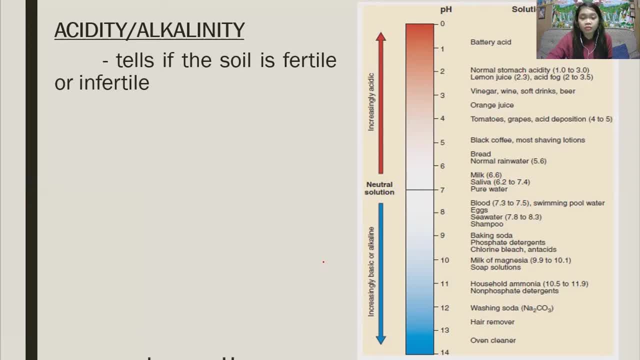 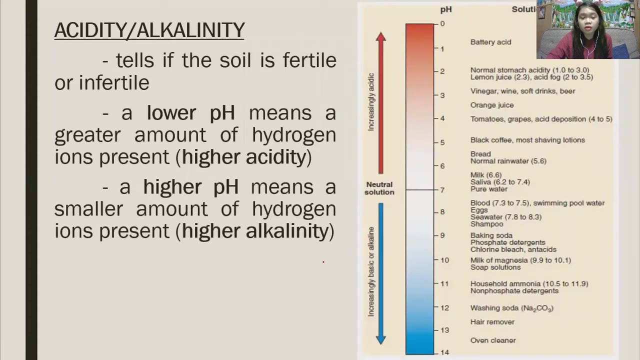 or also not applicable for plant growth. then a lower ph means a greater amount of hydrogen ions present. so lower ph here means a higher acidity, and then a higher ph also means smaller amount of hydrogen ions present or higher alkalinity and then soil acidity or alkalinity. it helps us determine the available nutrients that affect the plant growth. so 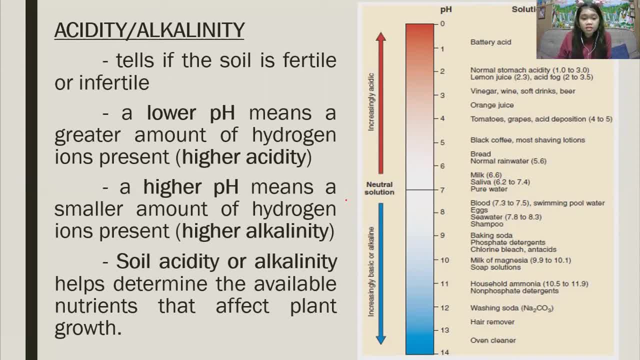 so, um, the levels of acidity or alkalinity is measured in this, in this figure here. so, uh, usually it's from zero to 14.. and this is the usual ph scale when divided from basic to acid. and then this ph reading indicates the reactive hydrogen ion present for the different types of soil, then this ph also is: 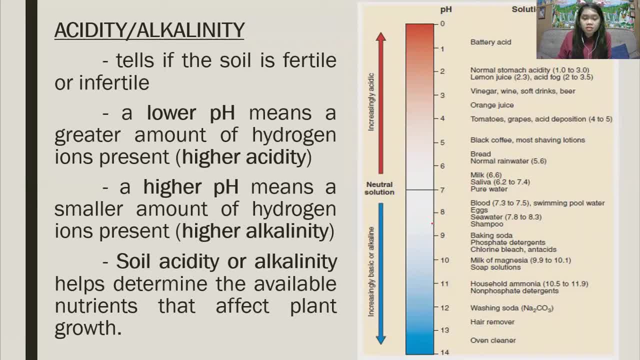 quite logarithmic, meaning that every changes, every changes in a whole number or whole ph number, represent a tenfold change also. so, uh, it is also an inverted, it is also called an inverted scale. so so low ph value indicate an acid and acid soil and a high ph. a high ph usually indicates an. 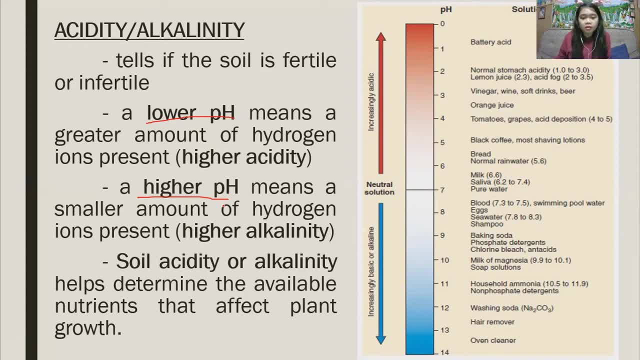 alkaline or basic soil. so uh, for usually for rainfall days, rainfall, heavy rainfall. so we have uh understood that the leaching process will increase. so it usually represents the soil elements, such as sodium, potassium, calcium and others with hydrogen. so so the desert soil soil tend to be more alkaline or more more basic, and soils in humic regions tend to be more acidic. 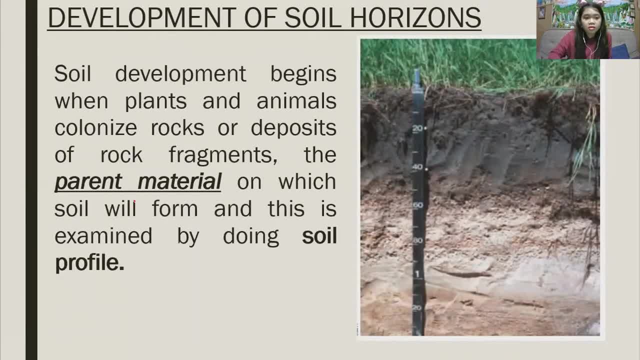 now we go to the developmental soil horizon. so, uh, soil development. so development begins when plants and animals colonize crops or deposits of rough fragments, the parent material on which soil will fall, and this is examined by doing soil profile. so so what we can, what you can see in this picture is that this is a vertical. 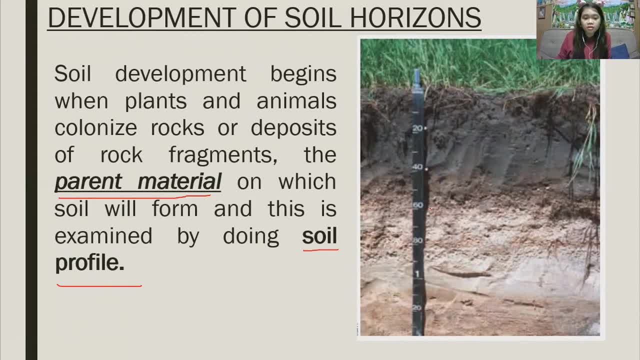 cross section. usually this is a vertical cross section of the soil from the surface down to the parent material. so when you say, uh, parent material, these are usually referred to as rocks, or or usually big rocks or big soils that are being being uh degraded, or in a long time. then, um, it results to work along the time, so so. 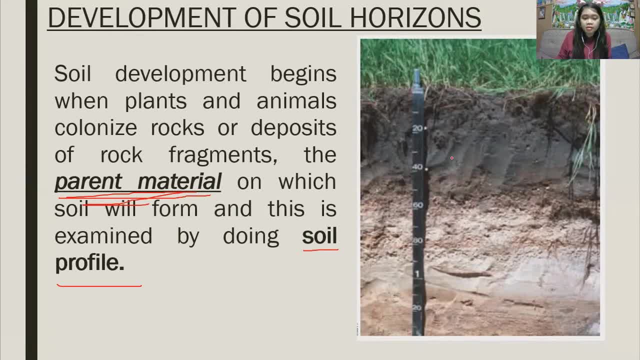 a soil profile here is used to examine uh the composition, the color, the structure of this type of of um parent material or rocks or deposits. they usually dig a pit by vertical walls to clearly show the different variations of those of those soils already, and then these types of soils are then used for uh what's called uh nitrogen management. so this is a 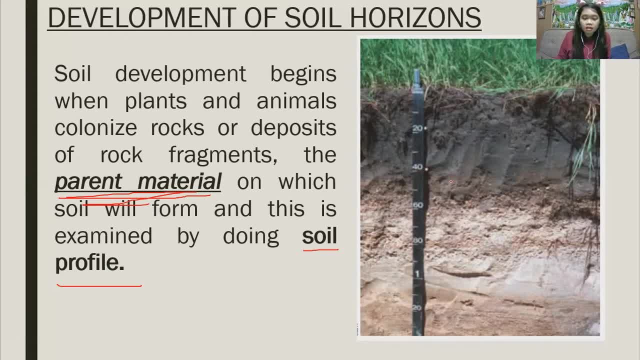 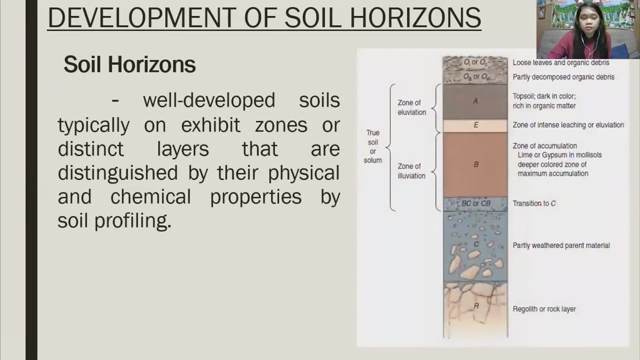 very important tool, uh in nutrient management, the soil profile. so by doing this we can gain a valuable insight about the soil fertility and the different types of uh, of uh, soil changes happens, so if, if it's applicable, that weathers and then the organic matter that decomposed. so here i will be discussing soil. 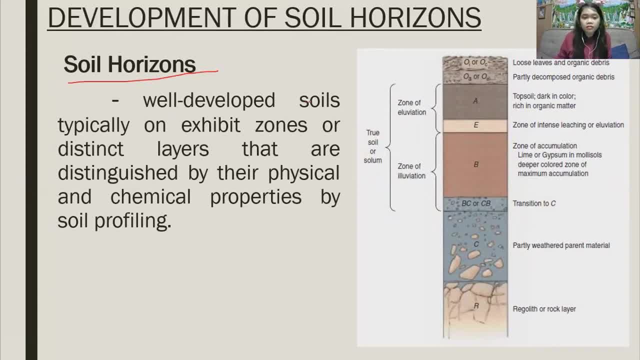 horizons, so well, soil horizons. these are the well-developed soils, typically on exhibit zones or distant layers, that are distinguished by their physical or chemical properties by soil profiling. so not uh, not just. they know the structure, the color or the texture and the composition of the 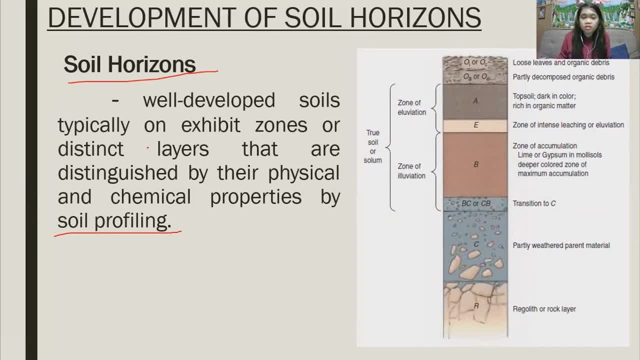 soil uh from the parent material. they usually they do usually make layers or study the different layers of soil uh, resulting in their soil profiling and that layers they have different uh. this can distinguish different physical and chemical properties. the soil horizons are usually designated by by letters. here they refer to their composition, to. 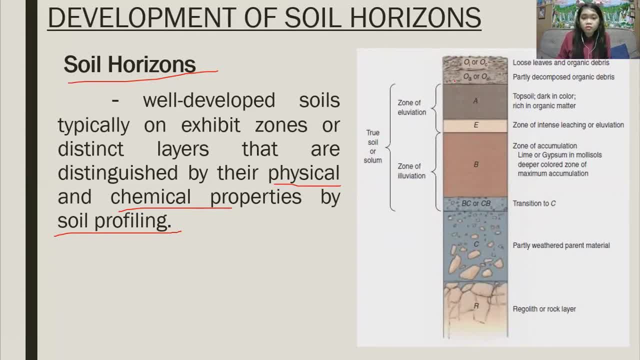 their dominant process and to their other position based, uh, soil profile. so we have here, uh, oh, we have the only horizon. so this horizon, usually the um, this is the layer sufficient for vegetation and moderation or moderate, and have moderate organic decomposition. so meaning is that they have. 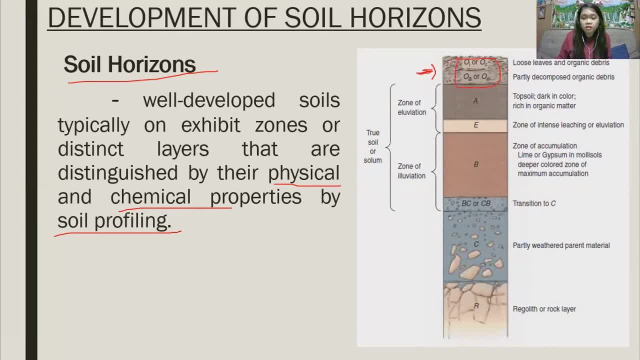 this layer of soil have a high composition of humus. here it's very rich in organic material. and then for a horizon- and this is commonly referred to as soil- they are dark in color and uh it's because of the concentration of the different uh decomposed organic matter they have. 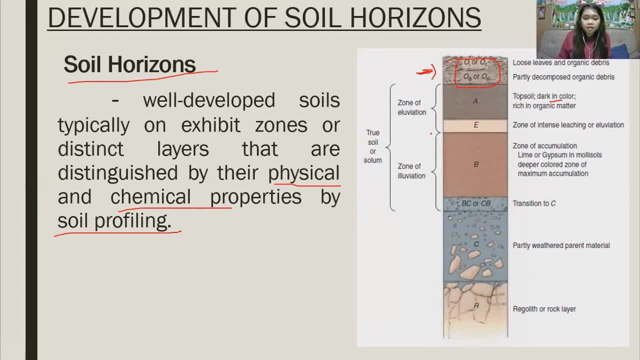 so, beneath the a horizon, some have a lighter colored soil. we have e-horizon, uh, namely after theachts process, um, the nutrients and minerals from the soil then, um, then the nutrients will go, So, especially the fine particles which are the clay and the silt, they go to be a small part of a deeper part of the soil. So E-horizon, here they are downward, They are the downward removal. There's downward removal of soil components between the topsoil and the water. 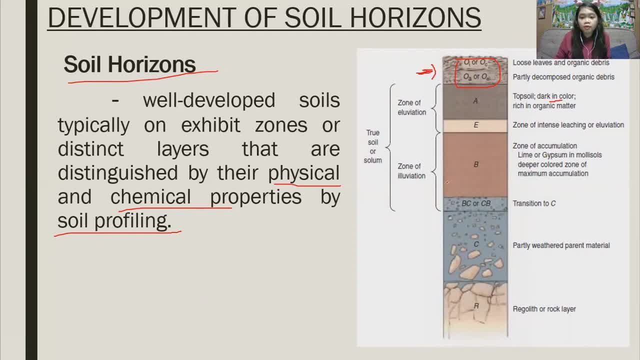 And then again for letter B, this is the B or C-horizon. here For B-horizon, this is the starting of accumulation of panacea, And so we have here lime or chitsum. You could find it here deeper in color zone than maximum accumulation, because the more lime or chitsum deposits here, the more darker, the more reddish it is. 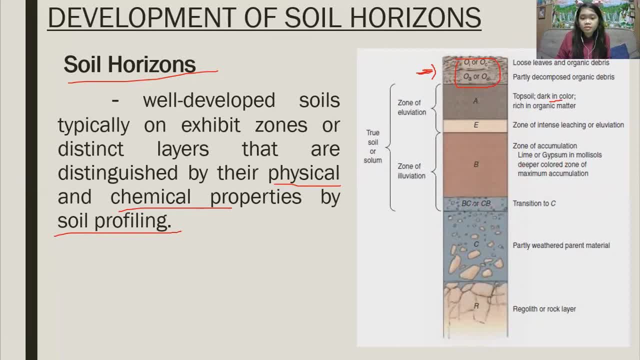 And then it starts in the transition of C- C here, C-horizon. this is the weathered parent material, partly weathered material, parent material from which the soil has developed, And it could be the different fragments of the bedrock directly beneath or below the rock, materials that had been transported or deposited. 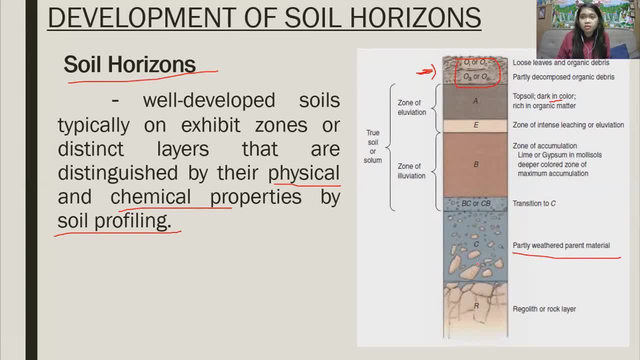 So, as I mentioned earlier, the parent material, These are the colonized rock and fragments, different soil fragments that are decomposed or nabungkab siya along the time. So we have also from the lowest layer there are or the regolith or rock layer. these are the unchanged parent material, meaning it never undergoes any colonization. 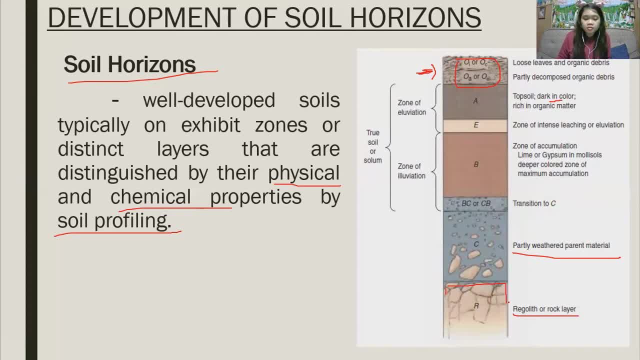 So it's either bedrock or rock fragments transported directly to the set of water by rain, glacial or other surface processes. So this process is that identifying the different soil horizons. this is usually used by soil scientists to determine the different physical and chemical properties of the soil. 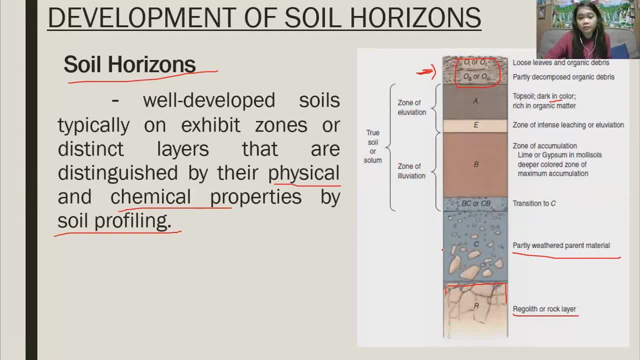 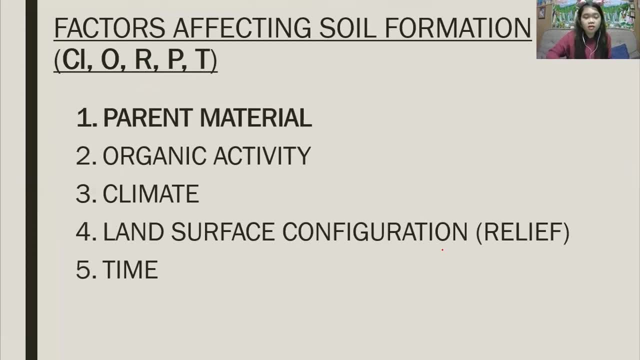 that they have conducted. so now we go to the different factors affecting soil formation. so the first factor here that we'll be discussing is the parent material, because this is the raw material of our discussion with happen on soil formation. so we have, we will also discuss organic activity, climate, land surface. 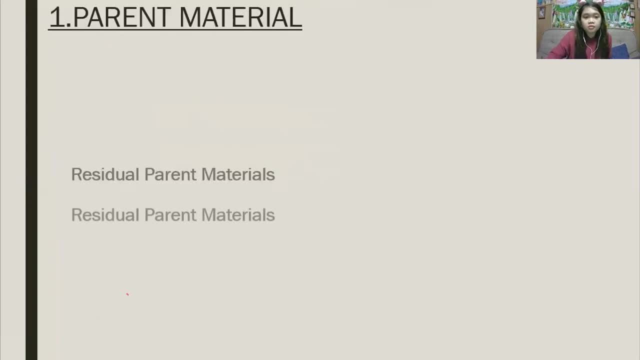 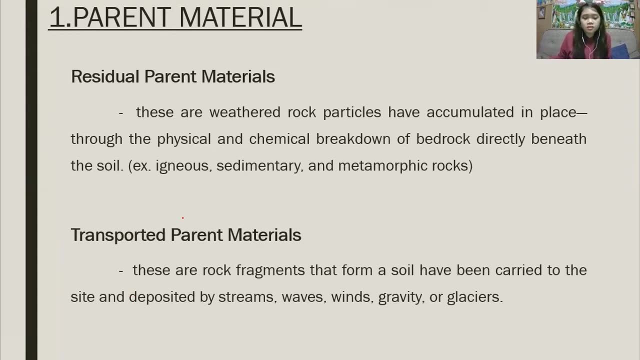 configuration for relief and for parent material. we have two types here. so usually soils are produced from rocks which are the parent material for the process of weathering and naturalization. so all soils contains a weather provenance material and it should be classified according to these two. so we have residual parent material. this means that there are, these are weathered. 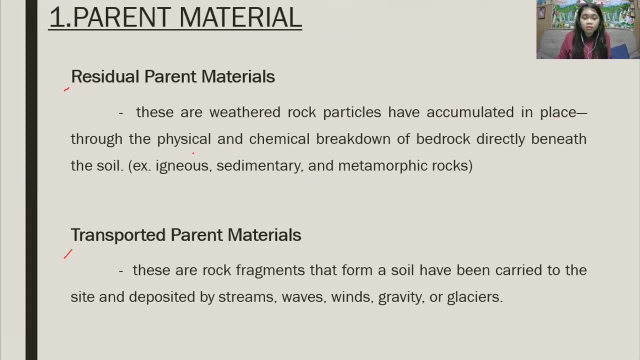 rock particles that have accumulated in place through the physical internal breakdown of bedrock directly beneath the soil. so when parents materials are usually break down at the same place and then look at the so that that is called residual parent materials- example for this are new sedimentary and metamorphic rocks. and then if we have transported their materials, this means that 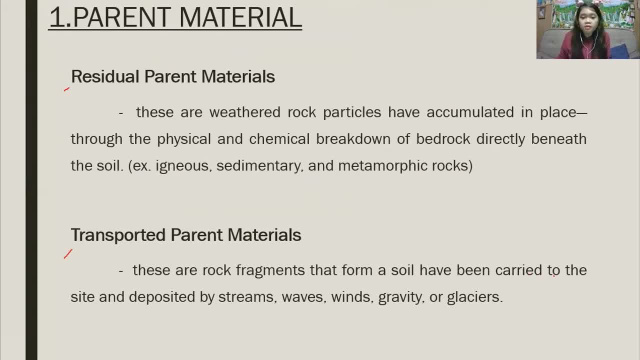 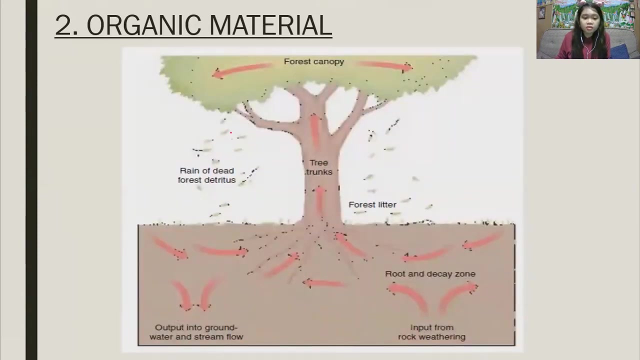 these are rock fragments that form from soil that have been carried to the site and deposited by streams, waves, winds, gravity or glaciers. so this is also a uh type of uh parent material that usually then we have uh organic material. so organic material usually, um, it is very uh. 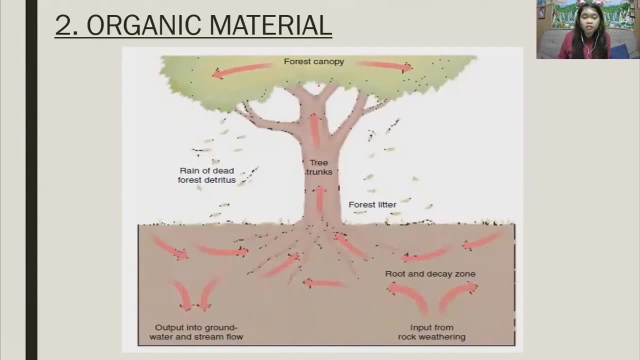 it affects the soil formation the way it can reacts, the way it reacts to the beneath the soil, uh to the plants, and then uh plants and animals. this affects self-formation because this organic material, like the organisms, uh they usually um give something to the soil and to the plants when they decompose, so so 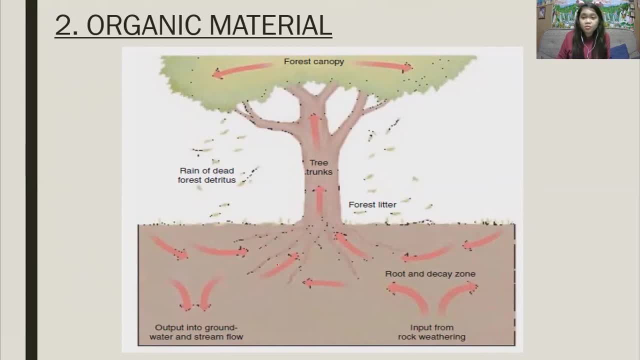 So for plants, magsubot na din na sila of growth. if there's a soil die. So as soil forms, plants begin to grow. And then, as plants mature and they die, new ones take place. Certain nutrients absorbed by plants. they are returned in the soil after the plants die and decompose. 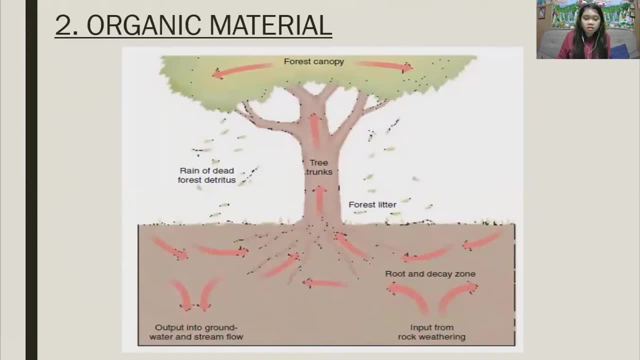 So after they die, soluble nutrients that are not used by plants can be lost through leaching, which can be used to improvise the soil. So that would be the very big contribution of plants. So when they decompose and die, they give nutrients to the soil to sustain another plant growth. 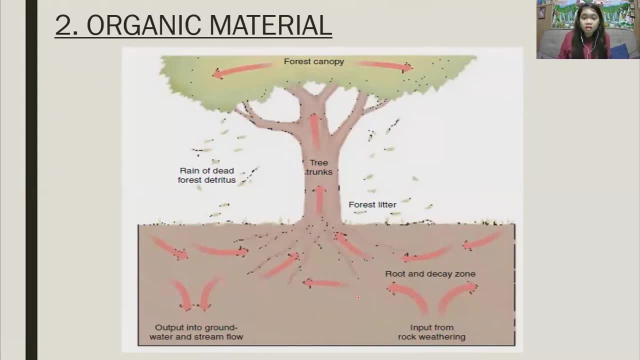 And then the nature of plant immunity determines the nutrient cycles that are involved in soil formation. Generally plants' forests- they have this term called forest canopy. Usually this canopy is a protective canopy to prevent the soil to wash out all the nutrients from a heavy rainfall. 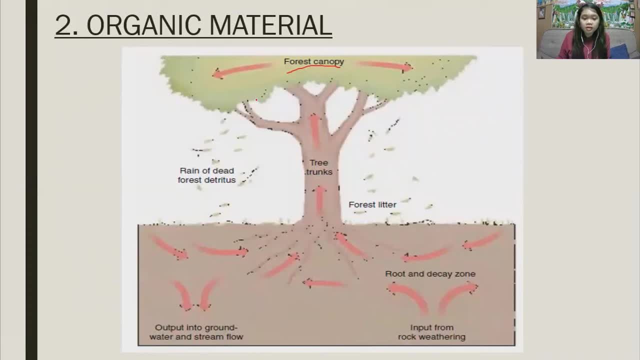 And then it keeps. It keeps rain from dripping directly on the soil, thus increasing the proportion of rainwater that enters in the soil rather than running off its surface. So it doesn't wash out all the nutrients in the soil because of heavy rainfall, if it's because of the forest canopy that is provided by the- usually the trees. 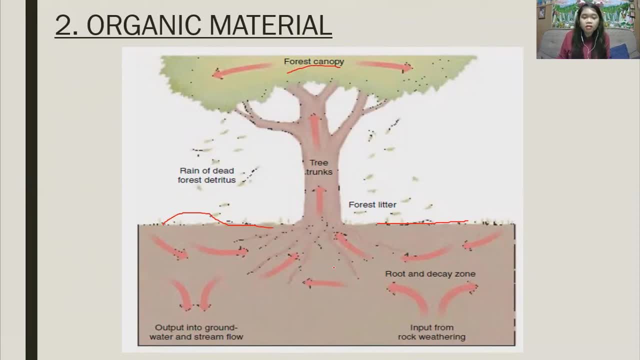 And then the microorganisms here, The, The fungi, the bacteria- they are the burrowing insects- and the animals, other types of animals, and even humans. If we die, the process of decay, the process of decay and decomposition, it's aided, mended by bacteria, right. 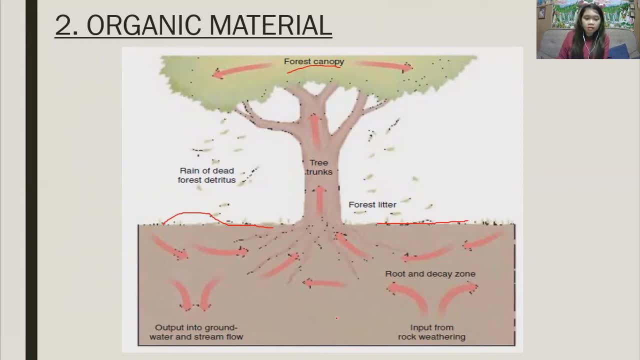 And from the activity. So it transforms organic matter. it transforms organic matter into a jelly-like mass called humus. So basically, humus is very important for plant growth. It's an important plant soil component for several reasons. For one, humus is a primary food supply for soil microorganisms. 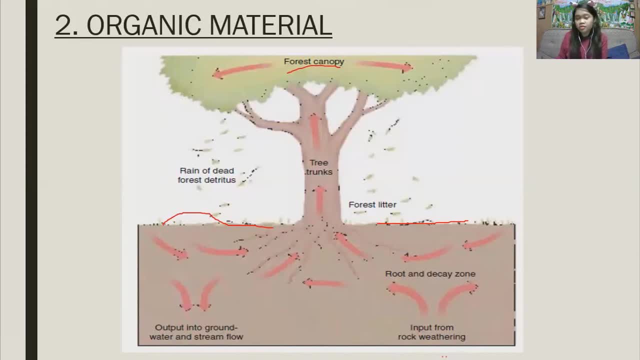 And without that these microorganisms could not live and could not execute their way of providing a sustainable growth. So organic material is a big part of soil formation because by doing so the plants and the microorganisms, they have different inputs for the 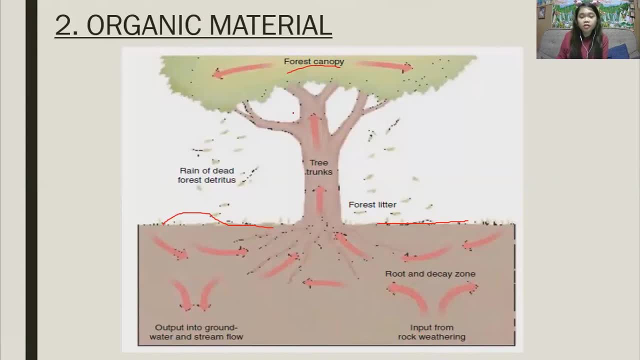 For the inputs for the different plants. And then, first, input is that through rock weathering, So they have, They have To achieve the decay zone, the diurn, and then the nutrients, which goes back to the plants, And then the output is the ground water and the streams that that flows in from the soil. 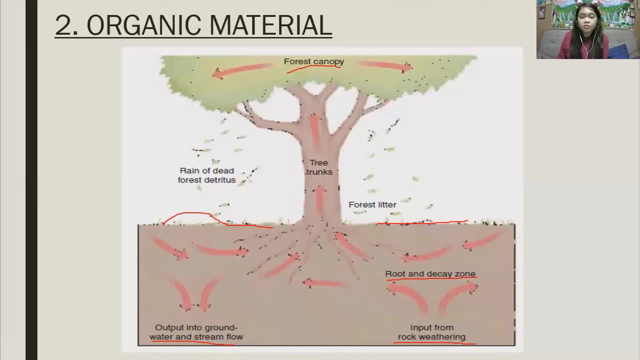 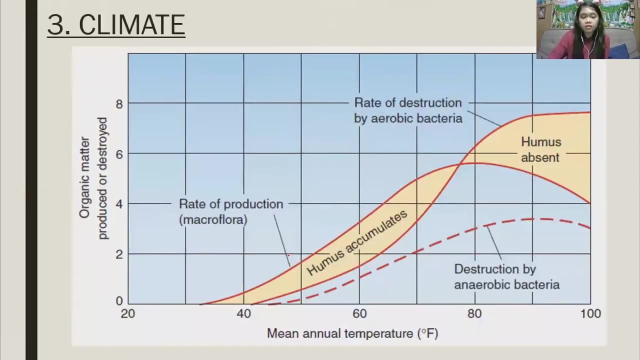 These are the. Also, some of these also are going to be plants to sustain life. So that's how organic material could, Could, Could affects soil formation also, for climate it's also one of the major major factor for soil formation because temperature directly affects the activity of the soil microorganism, so which this inference. 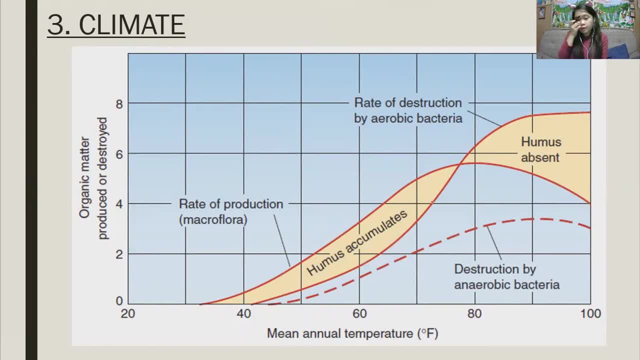 affects the rate of the decomposition of the organic matter. so here in this diagram uh in usually in hot, in hot region, so in high places, intense activity also. microorganisms preclude thick accumulation of organic debris of humus. so so, um, uh must have uh microorganisms that could uh use humus in happy tutorial legion, so so 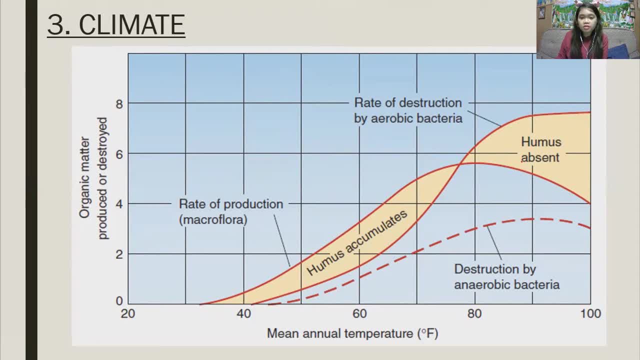 uh because because uh, there is a a high temperature, it limits, it limits the uh rate of destruction by aerobic bacteria. and then, in cover region, the combination of regarded microorganism activity and limited plant growth results in clean accumulations of organic matter. that may be, that may be either partially. 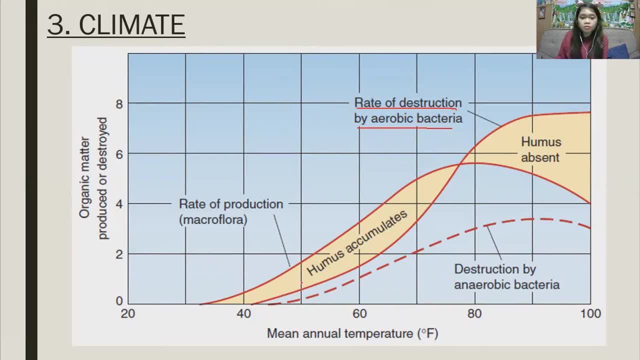 affected by decomposition. so here as the, the um, as the temperature is increasing, then after a while, if, if so, there's a faster rate of destruction of aerobic bacteria, those bacteria that have uh used oxygen for living, and then um here also for uh, the decrease would um. 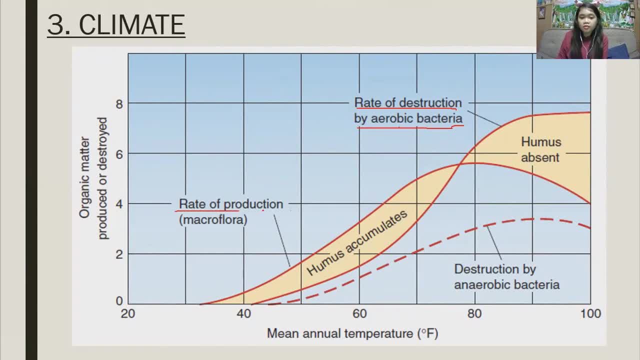 aerobic bacteria and then the rate of production of macromoflora. it's like it's a type of bacteria also. it's also increasing in as well in mean temperature. then it also starts to decrease as the mean and welcome picture also starts to increase. So the climate is a very big factor for soil formation. 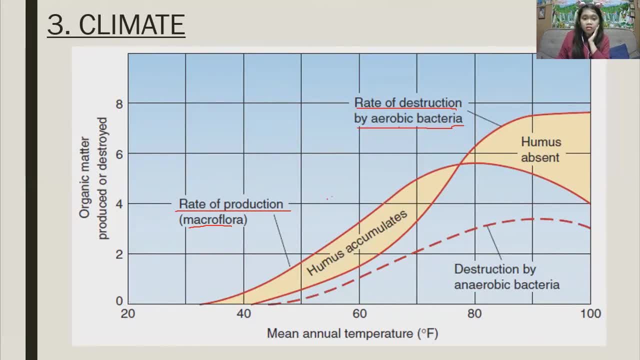 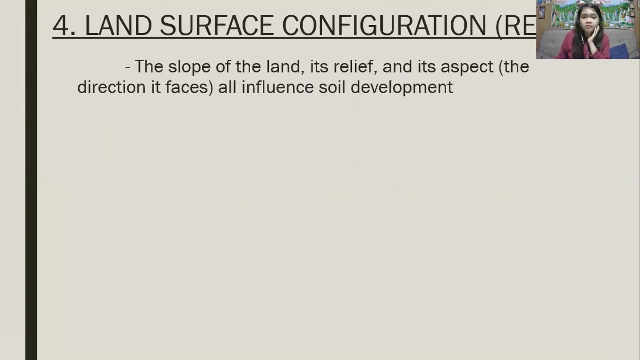 It shows the amount of organic matter and humus in soil increases toward the middle latitudes and away from the tropic regions. Also, we have land surface configuration, so it's also called relief, So the slope of the land or relief and its aspect. it refers to the direction or even 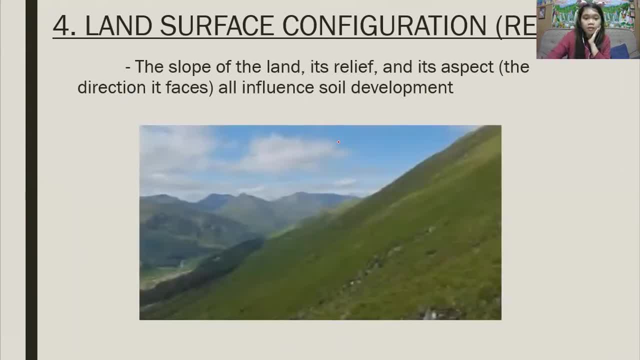 the direction it faces, all influence the soil development. So here this is an example of steep slopes. So steep slopes, usually they are better drained than gentler ones like a straight slope, Because steep slopes they are. They cause less infiltration of water, which retards in soil forming processes. 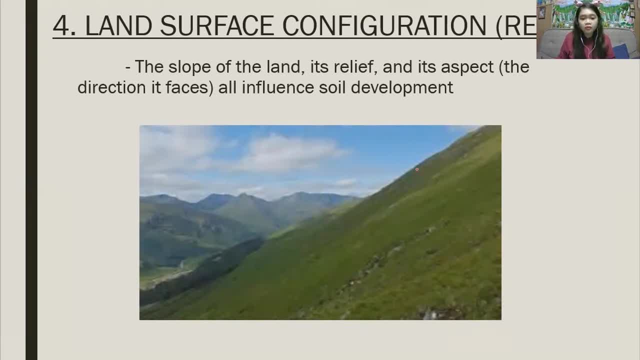 There's a rapid run-off of steep slopes that can erode surfaces as fast or faster than soil ever developed in them. So there is no soil that will develop on the parent material. in this type of land surface configuration. It's much less underdeveloped. 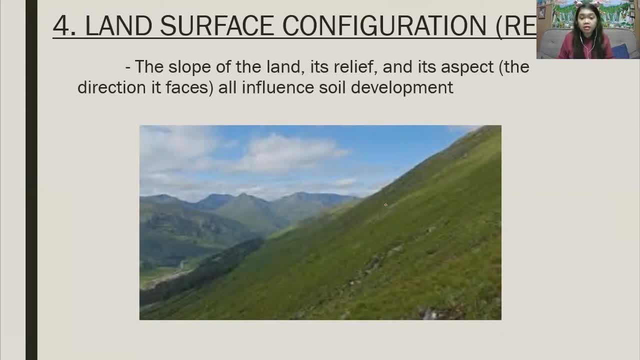 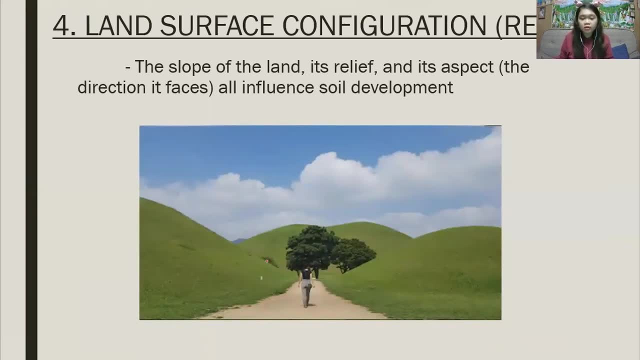 It's much less underdeveloped. It's much less underdeveloped in the development of the parent material For gentler slopes. it has less run-off and more water infiltration, So more water is available for soil forming processes and to support vegetative growth. 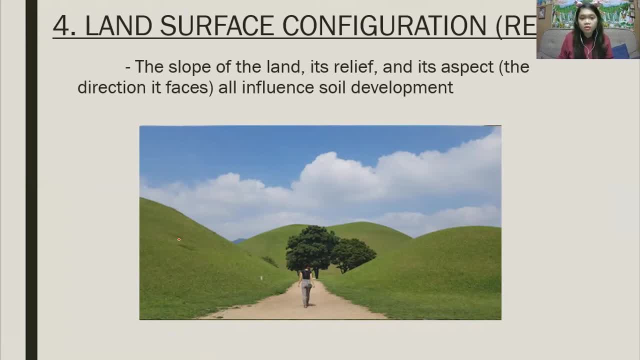 Erosion also is not that intense in this type of land surface or the gentler slopes. So there are different possibilities. The possibility that soil can form the parent materials that is associated in this type of soil earlier Surface configuration is faster. 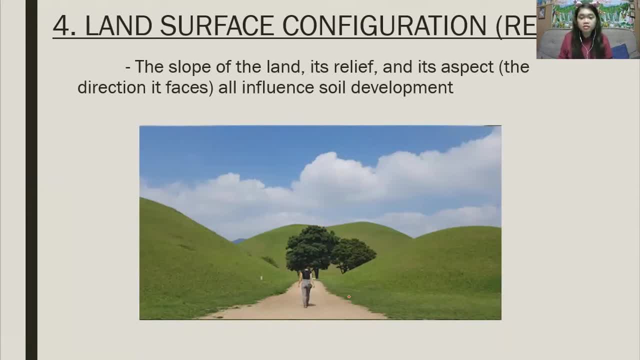 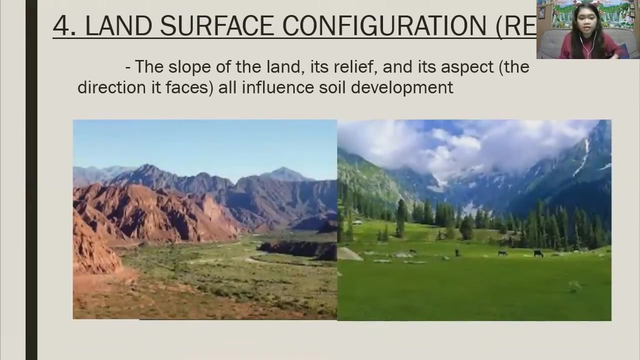 Changes are faster on the land surface. for gentler slopes with higher mud, Possibility to form permaelon. Possibility to form permaelon. And so those are soil from different parent materials. Also flat plants as well. Here we have valley floors and flat 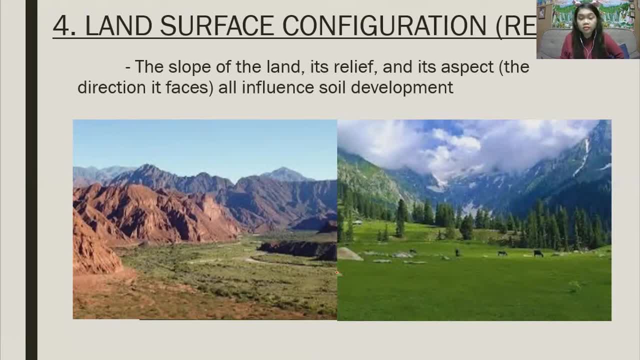 plants, So valley floors and flat plants. they are usually poorly drained because gravitational water from the rain cannot flow downwards Capillary water or the soil water. they could move harmful concentrations into salt and alkaline substance to the surface. So this condition. 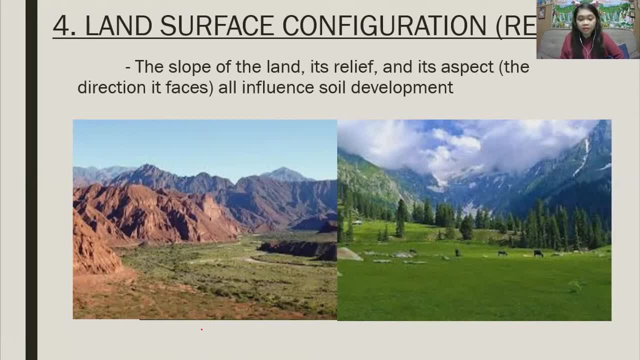 presents a constant problem for emigration. for flat plants They usually use drainage ditches here to support but to provide to lower high water tables in such instances. So in this type of land surface configuration it's very difficult to raise the water and this type of soil configuration is very difficult to influence soil development. 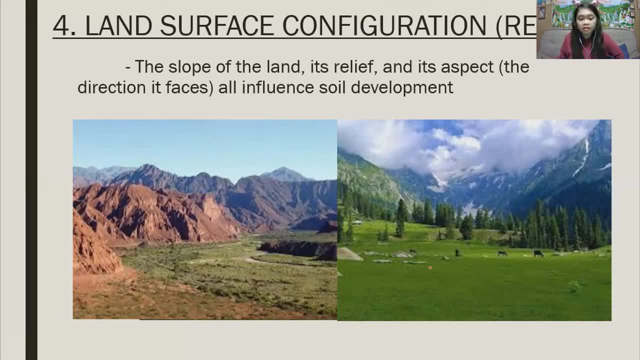 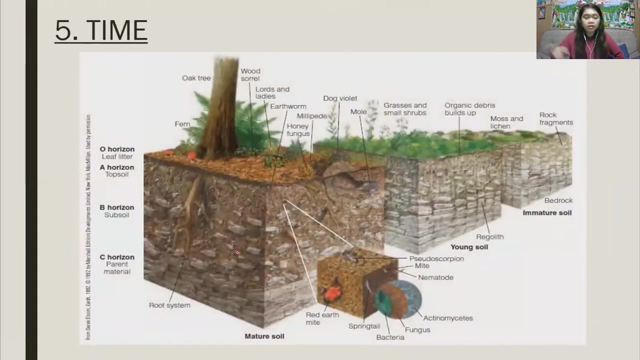 Land surface configuration indirectly can affect or influence soil development by vegetation, by the features of vegetation, because steeper slopes, they prevent the development of mature soil and that would support abundant vegetation. Here the last part is the time So soil have the tendency to develop towards a state of equilibrium. 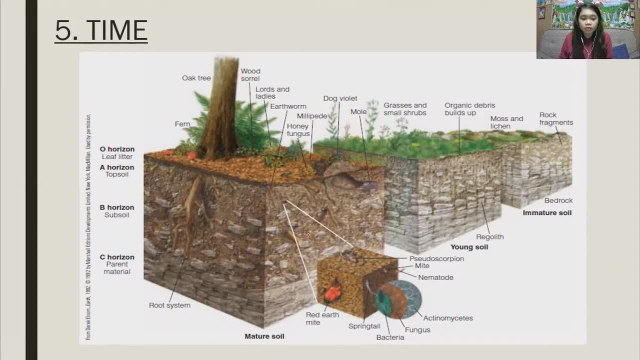 with your environment in time, So the soil becomes more mature when it reaches this condition. So we have here young soil that are still in the process of alteration to achieve the equilibrium, meaning the process of entering the matter and energy in the different forms of these soils are not that dilipakayushay. 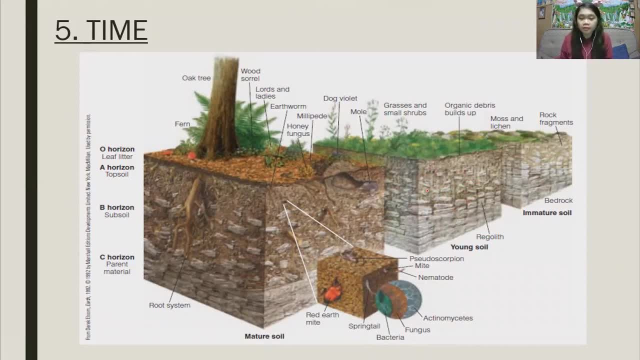 abundant. so here organic material accumulates as plant and other organisms die. so for young soil, that's the only thing that they could. they could do. they could do to achieve the equilibrium, or for mature soils. for mature soils they are well developed and stable horizons that 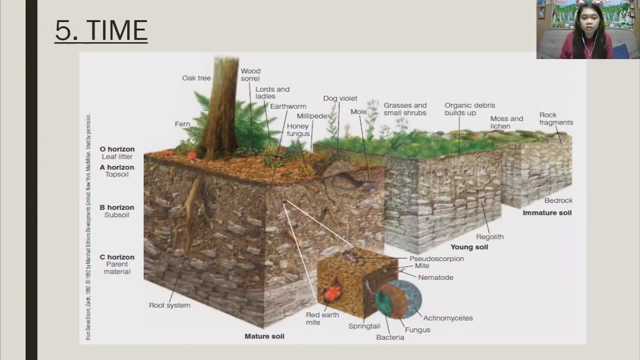 indicates the growth in the conditions of proper vegetation and plant growth. so they we have seen here that they contain greater amount of of organic materials present as compared to young soil. then for immature soil, these are typically poorly developed horizons and and my possibility, the parent draft here- is whether 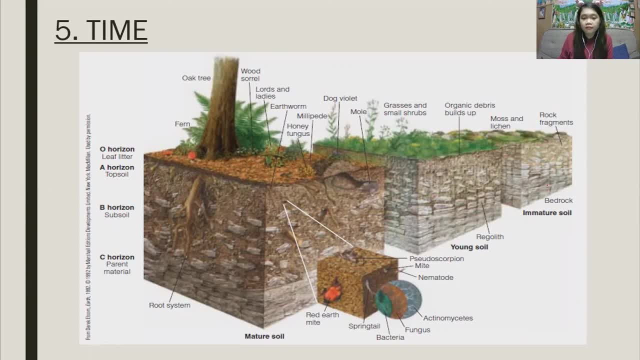 and the fragments for the parent material have been moved upward. that cause uh presence of of more uh bedrocks or rock fragments. so what are you guys like? process of organic material and other nutrients or minerals to support plant growth? another effect is that as time, uh, as time passed, 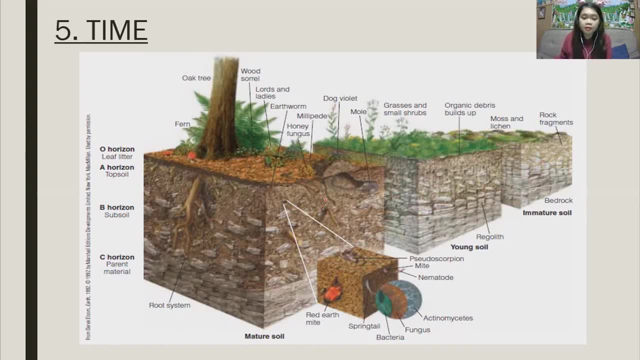 like all soils, were matured but their influence in the parent material decreases and they increasingly reflect their climate and vegetative environments. so my possibility gap on that young soil will mature at the certain period of time. so the time of developing the soil is an important to its composition and physical physical character. so given enough, 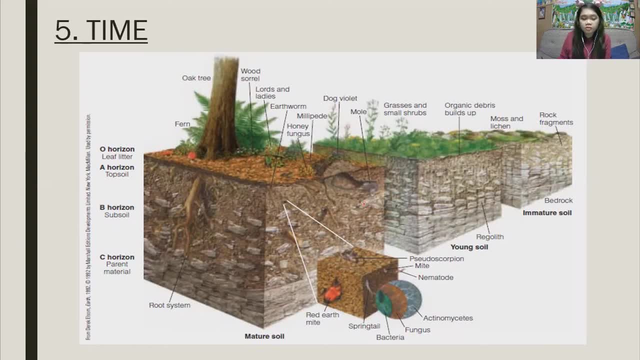 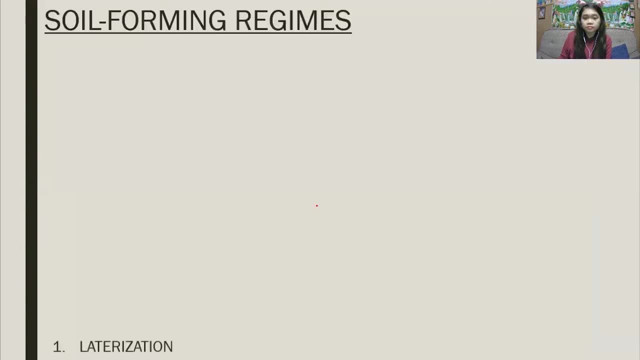 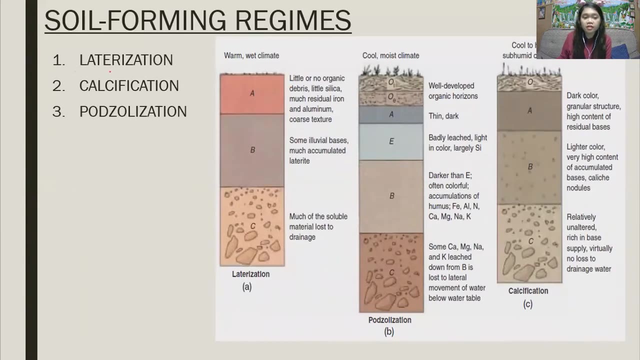 time and proper environmental conditions, soil will become more maturely developed, with deeper profile and stronger horizon development. so now we go to the different uh soil farming regimes. so we have here the lateralization, toxification and the fossilization. so the characteristics that make major soils type distinctive and other types distinct or they are different from each other, is to the soil. 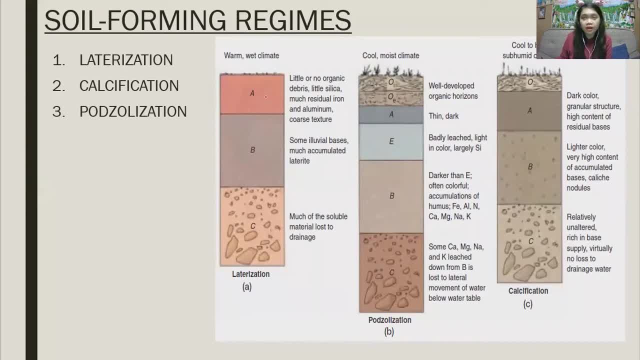 forming regimes. so these soil farming regions vary mainly because of the differences in climates and vegetation. so climate differences, where they produce three primary soil farming regions. we have, as i mentioned earlier, lateralization, classification and localization. so lateralization, as depicted here in the first picture, uh, it occurs in unique tropical and subtropical. 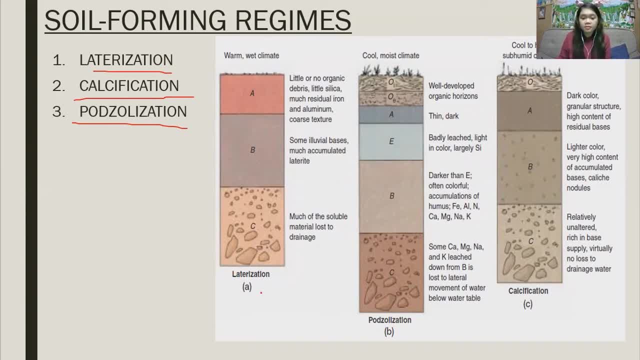 climates as a result of high temperatures and abundant precipitation. so must have done times in this other, because lateralization in this area. so it is a weathering process by which laterite is formed. so laterite, uh, laterite here is called soil or rough type that are rich in iron and aluminum. so 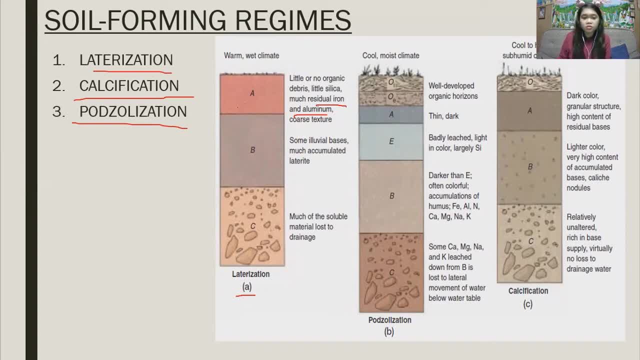 so in this process, soil and rocks are depleted into small soluble substances. so, and then we also have a process of fossilization. so fossilization here- i think i've mentioned it earlier- the soil horizon, they have the same, uh, they have the same process. so so this is the, the soil with. 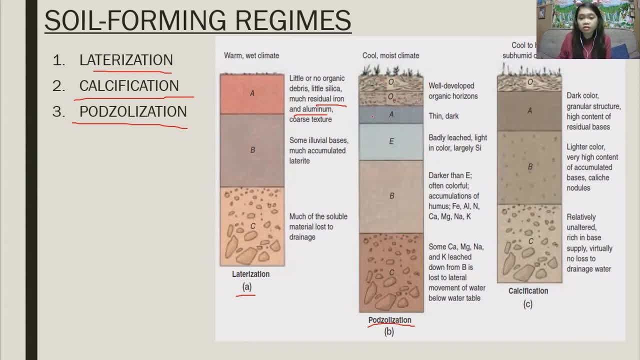 more rich of of organic material, more darker. here is the produce by the process of elevation. then here is the process of of uh, the after elevation and then um. fossilization occurs mainly in high angle latitudes where the climate is moist, with short and cool summers of long um long winters, and 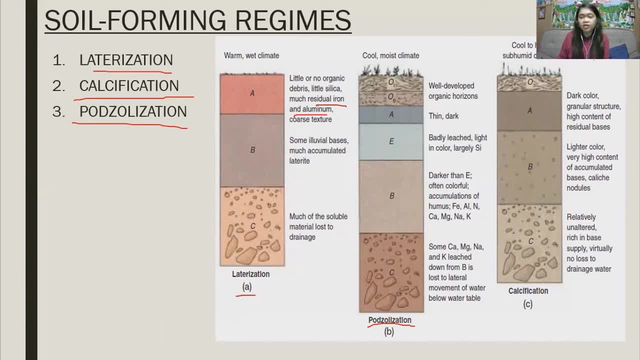 severe, uh kind of cold areas geared. so so this is the the formation of the soil if for cold to hot or sub-humid climate. so so this is the process of precipitation, so we could produce a a much more dark color, uh type of soil for a a horizon then. 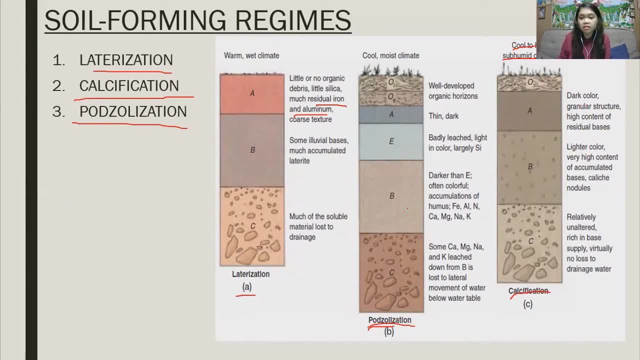 for the horizon, like their color, but not that light as compared to uh warm and and cold or moist climate. then also to see here the parent material, know weathering of parents materials. they are, uh usually unaltered, so below the ground in this type of of climate. so 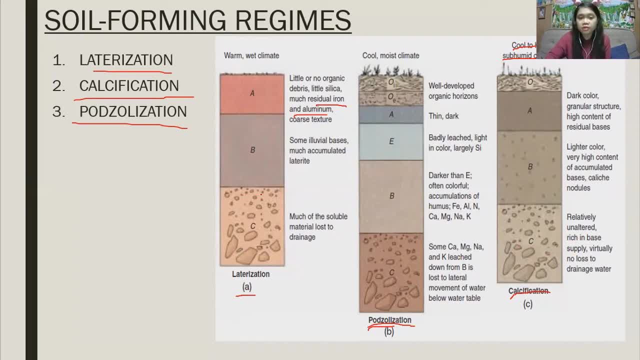 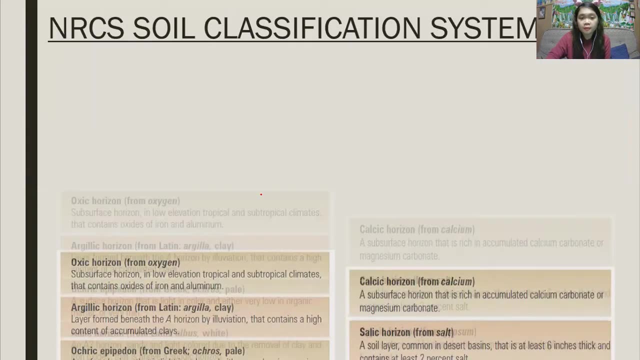 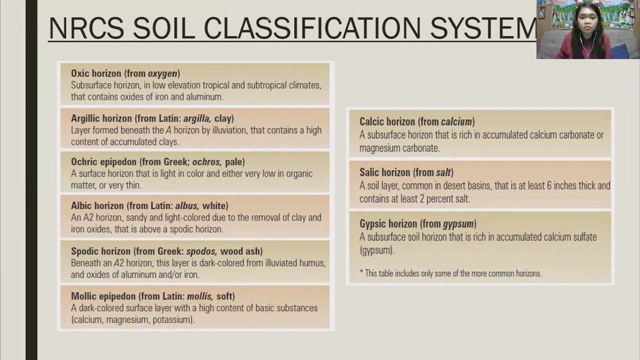 these are the three major types of of uh soy farming regimes. so we also have additional salinization and glazation that we will be discussing more on this either other lecture. now we go to the uh ncrcs soil classification system. so we go to the process of classification. 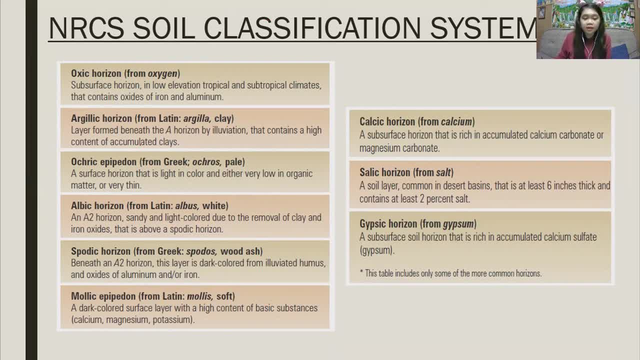 of soil, so soroads. like linux, they can be classified and mapped by their distinctive. we are, i mean process, they are service, they are results from surveys published in books already and it could help us describe the kinds of soil in a certain regions, and usually it includes maps that show. 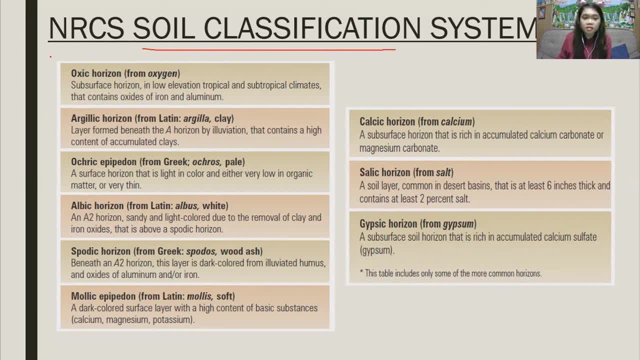 distribution of soil types in the us setting. we will be discussing the us. so they had this system called nrcs, where nrcs stands for natural resource conservation services, so it's a branch of department of agriculture in the us. these are the 12 largest classification of soil that they have. 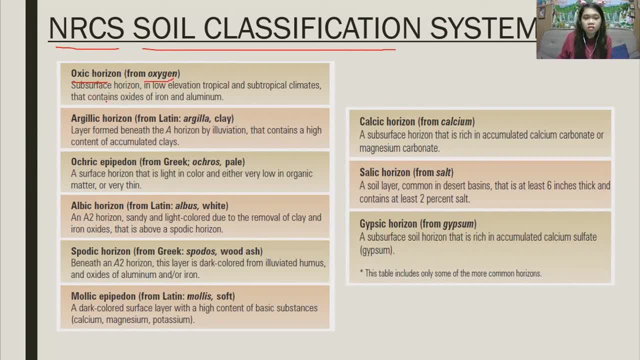 we have oxy horizon, rich in in oxygen. so, um, we will not be discussing all of this, but we will be mentioning sigoro here in the later slides. some and then um, and then uh, also um, while examining the soil for classification under this system, a particular attention usually is speed off. 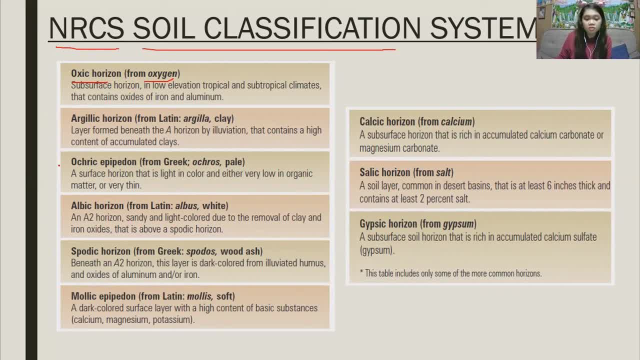 paid to the horizon group by its texture to characterize the soil. so some of these horizons, uh, are below the surface. so when you say below the surface it's, it's in the subsurface horizon, and then others are some of the epipedons, so epipedons. 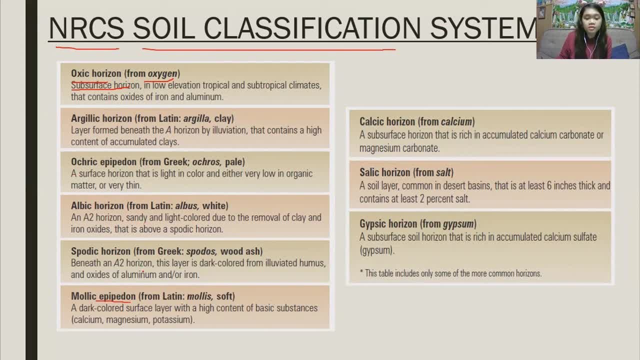 are here. these are the um surface layers that usually exhibit a dark shading associated with organic material or humor. so this is mostly the top part of the layer soil. so this classification also are um. they are classification of soils according to the soil order and then they can be given 12 that are recognized. so to provide a greater detail, soil orders or 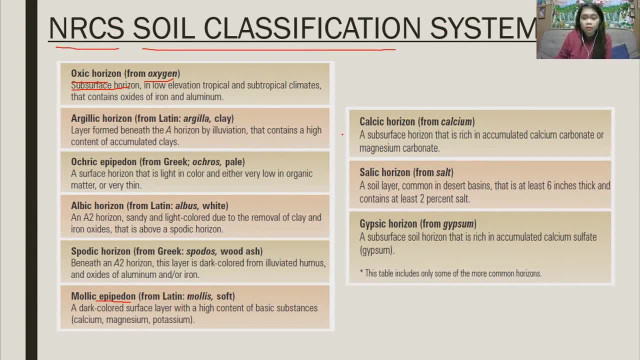 this soil horizon can be can be divided into sub orders and other groups, subgroups or families. so these are the animal. this are the 12 uh soil classification systems provided from the book. actually this- there's nine along the eye here, but uh, the other uh. the other three is not provided in the book, but you could. 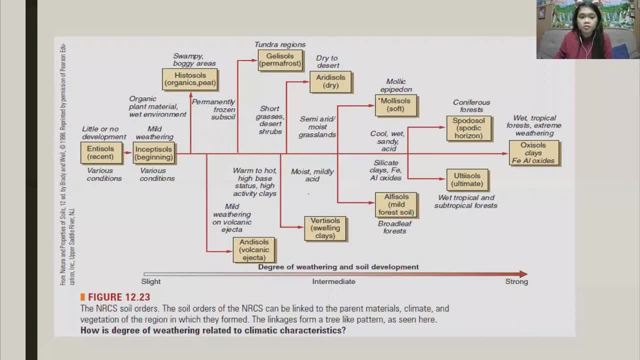 you could research more on it. so now let's go to the um 12 for the ncrs, for um, national natural resources, the conservation services specification system. so just we'll be just a short introduction on the 12 before we end. so we have here the infusos. these are soils that 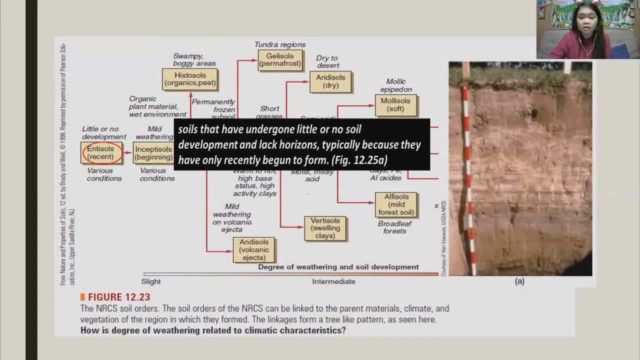 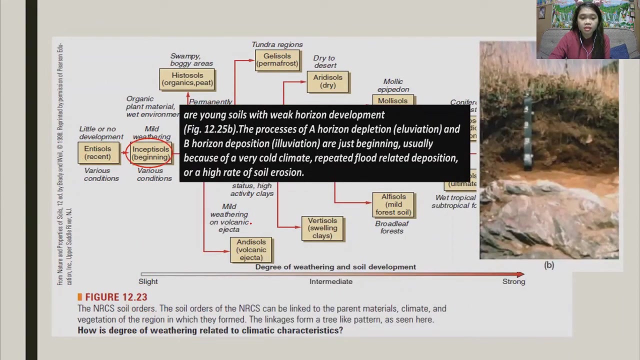 have undergone little or no soil development and halak horizons, typically because they have only recently begun to form. so usually these type of soils are very recent to mature soils with no abundance of nutrients, organic material presence, so usually they are the very material characteristics. so here we have next is in septic, also for inceptive sources, are young. 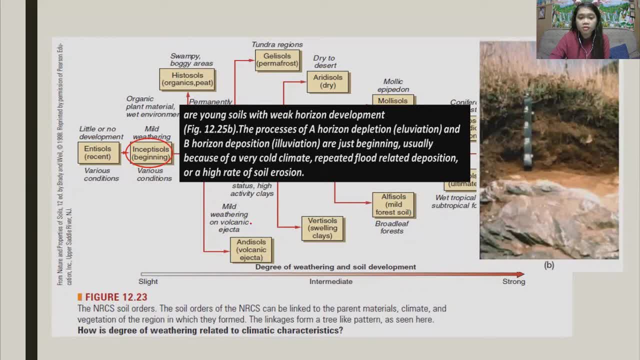 soils with horizon development, how the processes of these in horizon depression or the illumination and just beginning. so usually because of a very cold climate, repeated flood related deposition at a high rate of soil erosion, so these soils have the weakest appearance of horizons among the layers. so 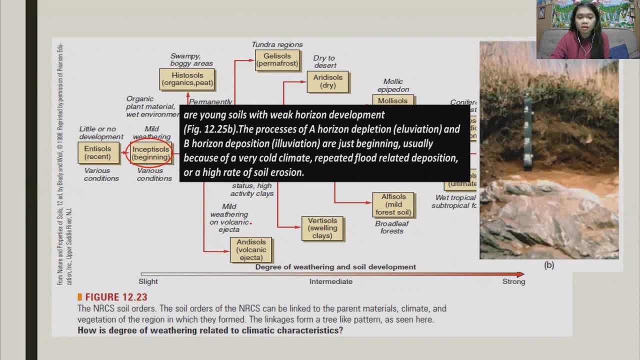 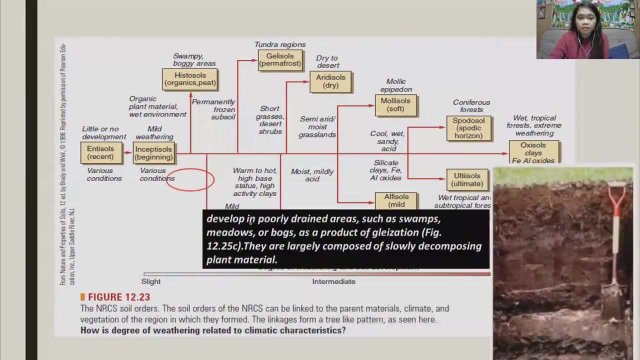 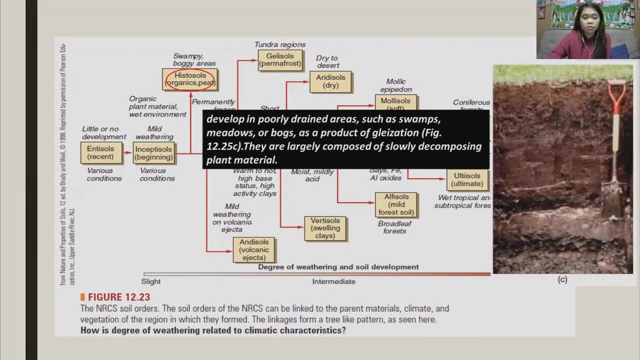 they are still soil forming types of soils. and then, and then they are also the most abundant in the earth, usually occupying, though, almost 22 percent of all non-polar continental land area. then we have histosols. so and histosols, these are a very low bulk density type of soil developed in 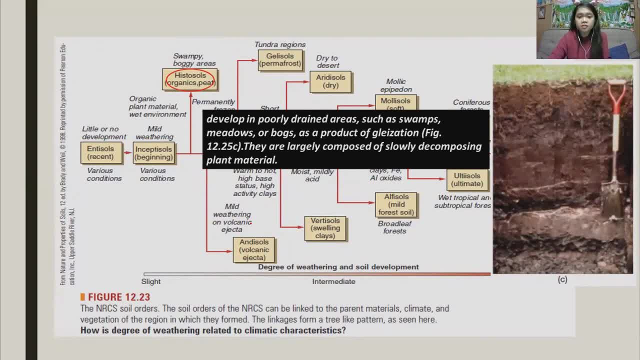 a poorly drained areas such as swamps, needles or bugs, as a product of radiation. so they are largely to photo slowly decomposing plant materials. so so in this process here, the nearly accumulated tissues of dead plants and animals that could uh possibly results to to the modest in this type of soil, and then um the soil like this have started to have. 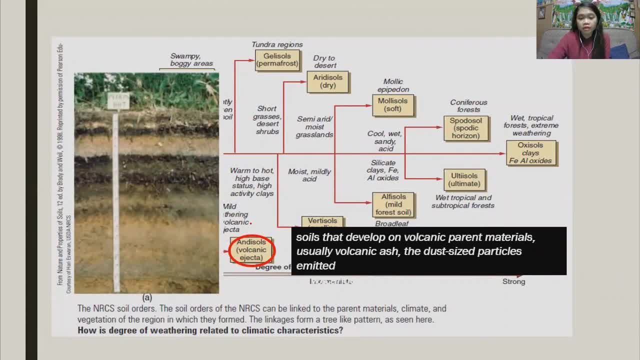 for under souls. this is also soils that develop on volcanic variant materials such that they require high organic content, materials such as volcanic ash and dust-sized particles emitted. so so these type of soils are? they are not very young. they are usually produced after volcanic eruption, then then volcanic ash. 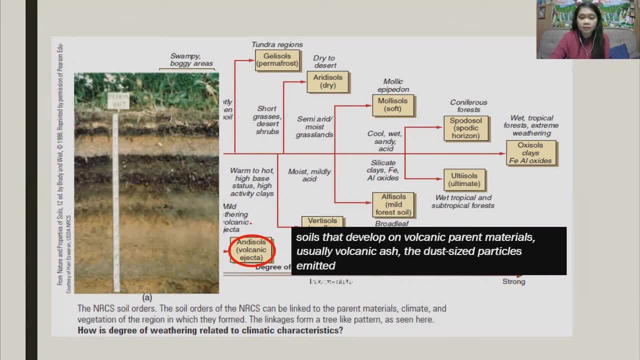 usually spreading, and then these soils are acidic, depending on what type of volcano they come from, and then they differ from those in other orders because they people, they typically are dominated by glass and short range uh order colloidal weathering products so such as the allopane. so that is an a characteristics of the undissolved- undissolved soils. 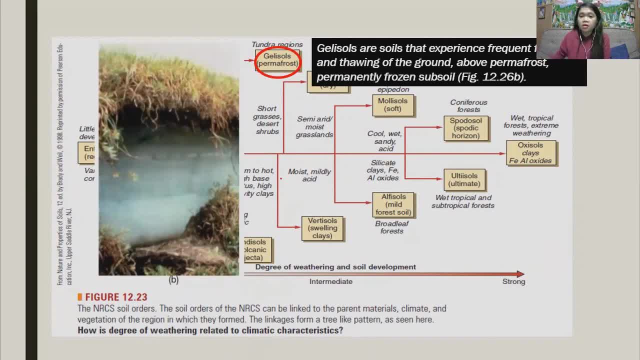 so we have gillisols. gillisols, these are soils are that are experienced frequently from freezing and thawing in the ground above permafrost. so permafrost, these are the the temperature of the soil ranging from zero degrees shoots below. so uh, the soil is canadian expressed or not introduced in this: uh, below temperature. 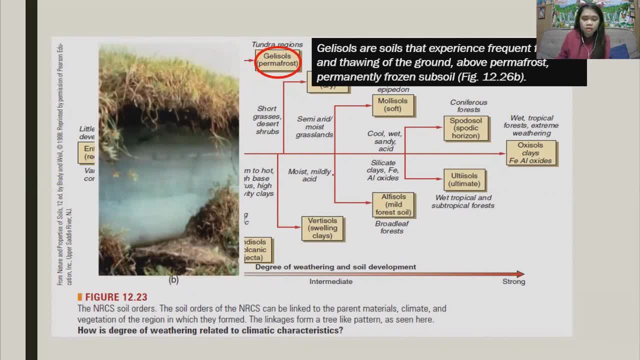 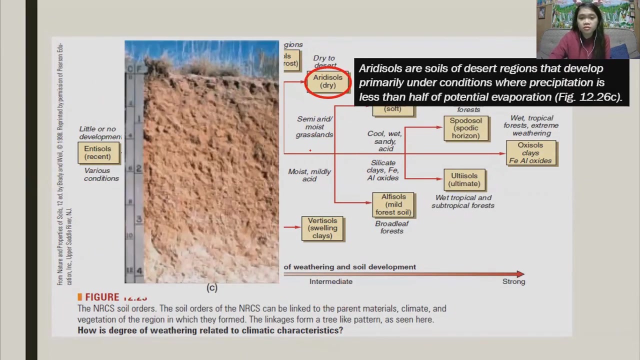 for at least two years and then um this was can be found in a very high, very cold climates, very limited, uh, geopolitically um setting, and then high latitude polar regions- we also have an already source, so these are soils of desert regions that develop primary leaf. 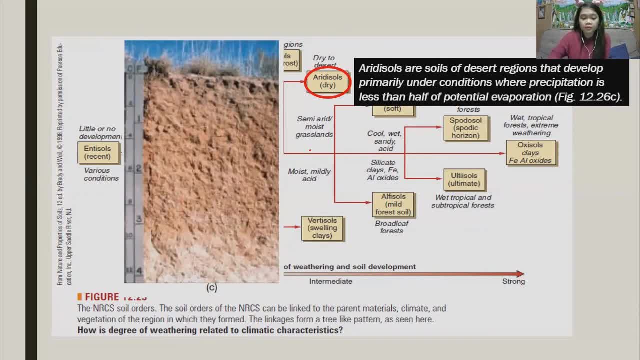 under conditions where precipitation is less than half the potential evaporation. so so light in color, a low view, most content: dry soil conditions. most a year, mostly a year, and then 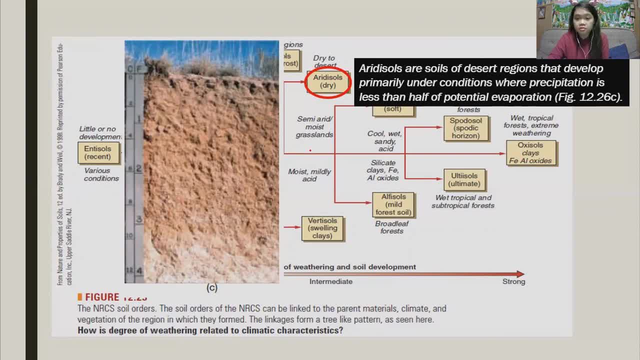 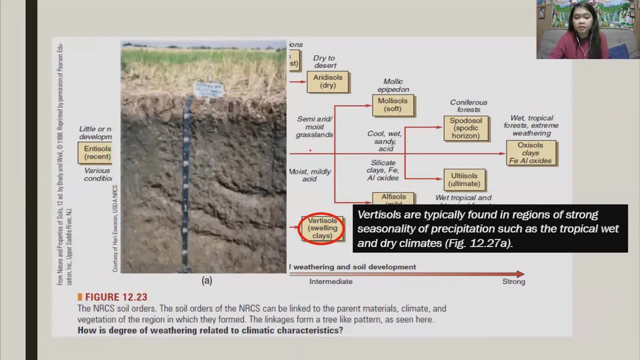 are known as desert soils for vertisols. these are typically found in regions of strong seasonality or precipitation, such as tropical, wet and dry climate, so here the species of soil have high 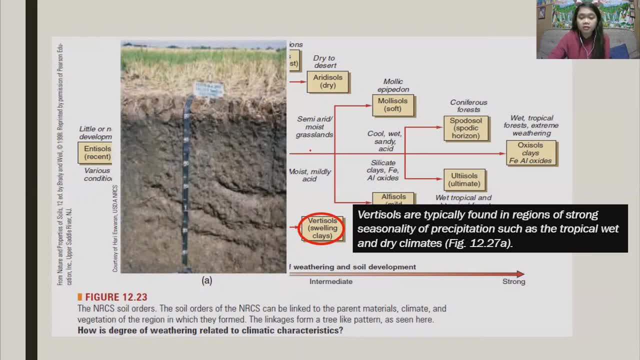 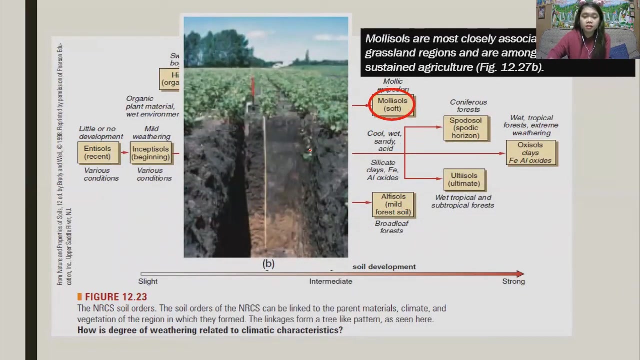 clay materials. and then they, these clay materials, absorb water and increase in volume when, when they started to form, dry, deep and and then much more darker type of soils- excuse me, molly soils. these are most closely associated with grassland regions and they're among the best soil for sustained agriculture. so, molly soils. 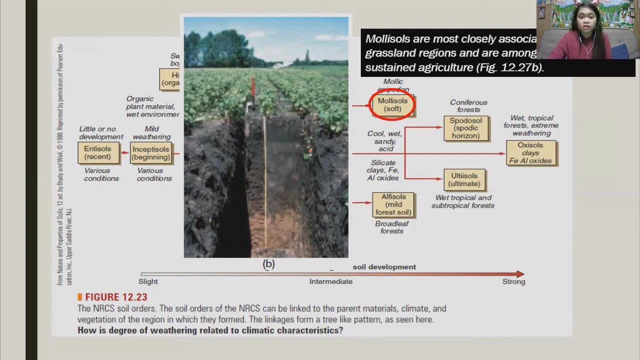 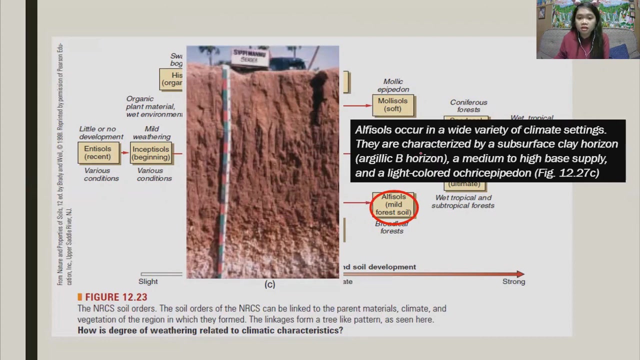 they are usually thick, dark surface horizon, fertile type of soil. they are long-term exposure for organic materials derived from plant fruits, so they are very or naturally highly productive soils, more than 50 saturated with calcium, magnesium and nitrate for altisols. they usually occur in a wide variety of climate settings. they are characterized by: 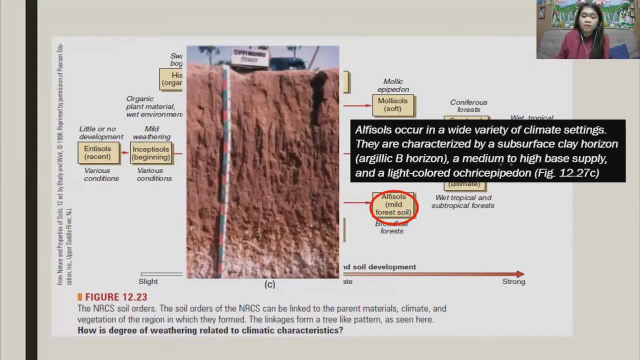 subservience, a subsurface clay horizon, a medium to high base of life and a light collared, sheer tartar typeMadça and an longer duration. 쓰는 question in the chat box. touched iPhone. let's hear that. go ahead, csto, okay. 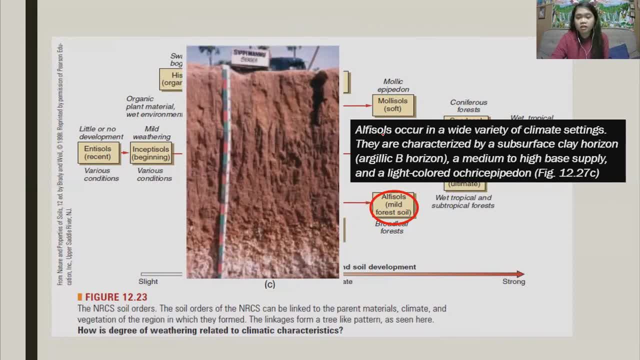 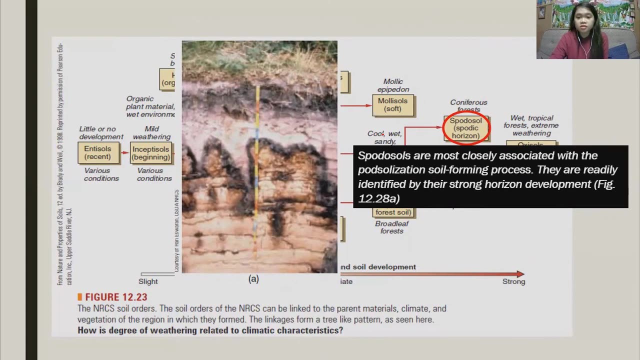 not. they are not uh appearing in this kind of area where there is very dry and in the warm places, usually in high, in a cold place, japon. so spodusos uh are mostly closely associated with the pulverization performing process. they are readily identified with the strong horizon. 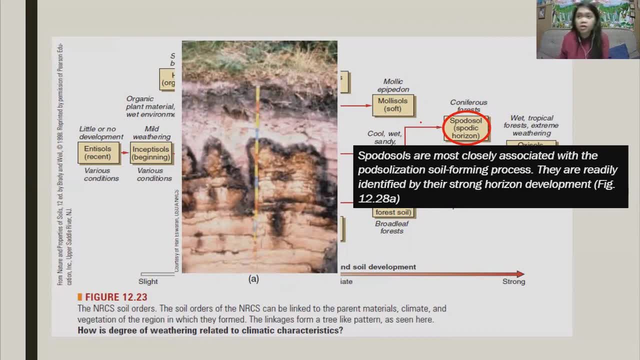 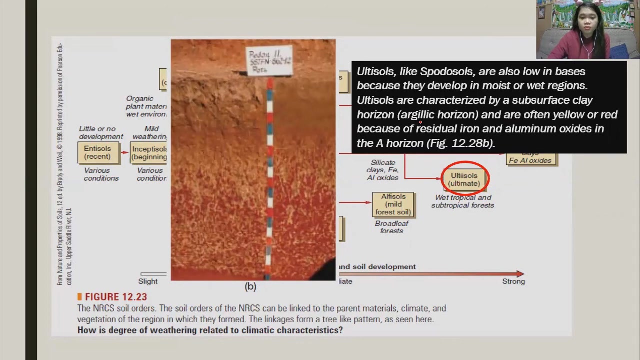 development. so when they say post elevation process, they have experienced television or nutrient reposition. so this type of soil are presence of organic material and they are also um, uh, subsurface accumulation of humus that is complex with aluminum and iron. so second, the last is also also like sputasols, um are also low indices because they develop in most moist or 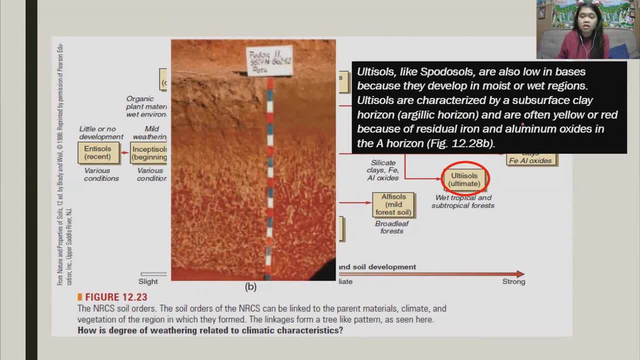 wet regions. so they are characterized by subsurface clay horizon and are often yellow or red because of the residual iron and aluminum oxides in the area. so basically, what you what causes the, the, the soil to be reddish type, is because of the iron and aluminum presence in the 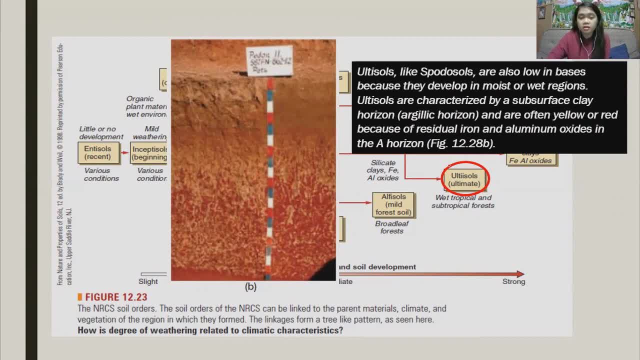 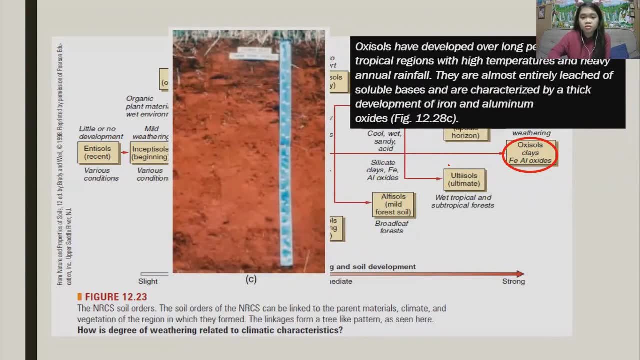 soil. so it's an example. this is the example of that, the reddish type also. so it's just the ultisols. and then for the oxysols, these are the the more developed soils over long periods of time. in tropical regions with high temperatures and heavy annual rainfall. they are almost entirely. 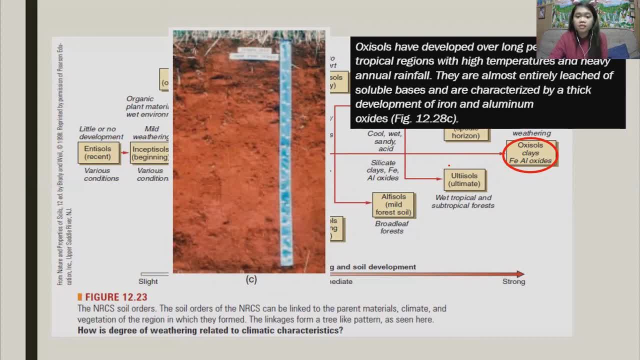 rich of soluble gases and are characterized by a thick development of iron and aluminum oxides. so the key basic profile characteristics of oxysol is that they are uniformly textured. they are, they have high amounts of iron and aluminum. reddish- japan color, and then they have